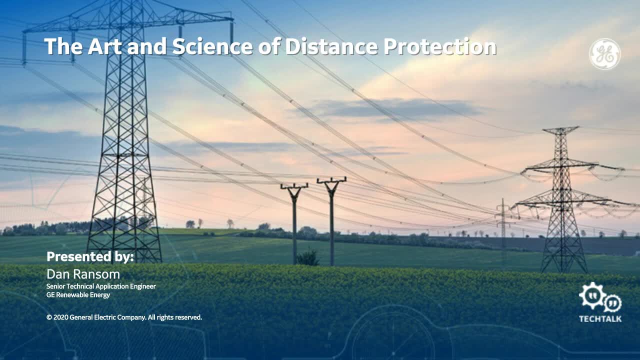 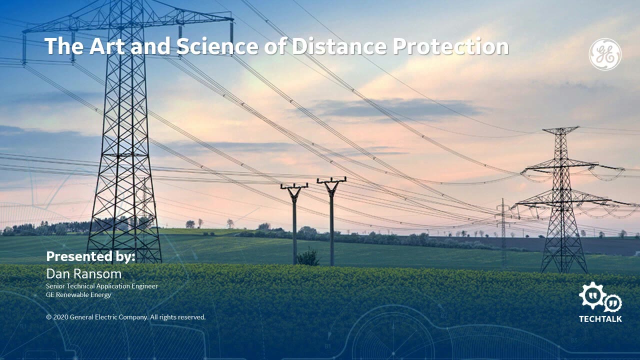 over to Dan Ransom, Senior Technical Application Engineer at GE. Dan, the floor is yours. Good day to you. Welcome to this webinar on distance protection. My name is Dan Ransom, Senior Technical Application Engineer at GE. Here's a little bit about me. I've 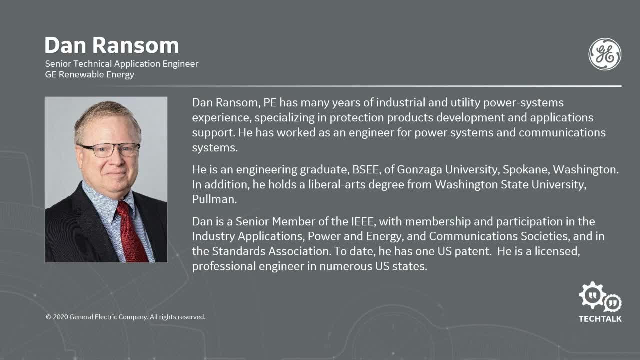 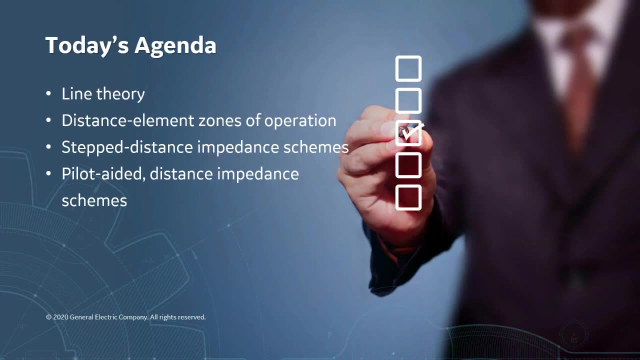 worked many years in industrial and utility power systems. I'm a graduate of Gonzaga University in Spokane, Washington, and also Washington State University in Pullman. I'm a licensed professional engineer in many US states. During this session, I'll discuss the following: line theory distance element zones of. 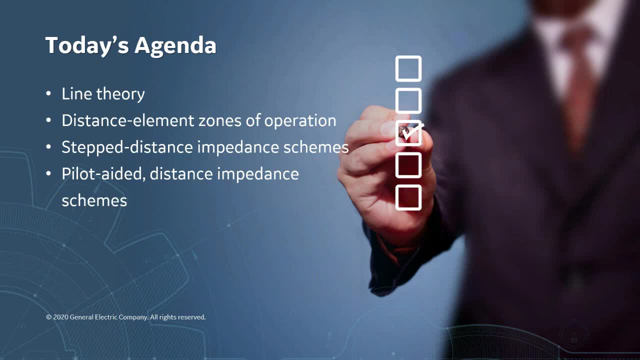 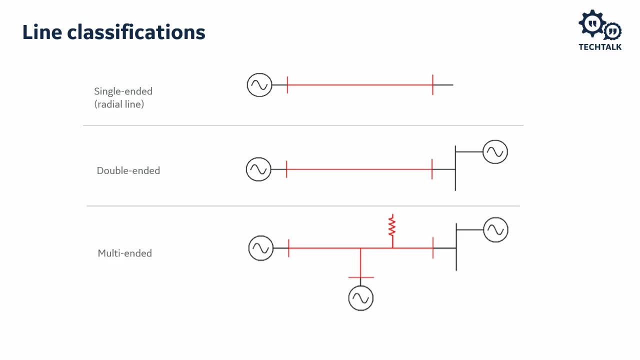 operation, stepped distance impedance schemes and pilot-aided distance impedance schemes. First let's take a look at transmission line theory. Transmission lines are classified into three categories that describe the presence of generation or possible sources of fault current that might be found at the transmission line boundaries. A single-ended line, also called a. 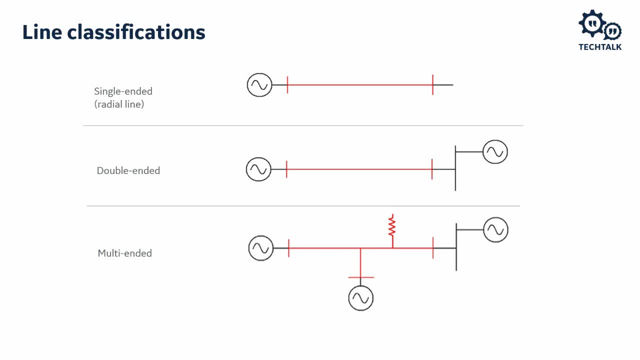 radial line has a source at only one end. This type of line delivers power from the source to a load at the other end of the line. Therefore, when a fault occurs, there is only one source of current to feed the fault. A double-ended line has only two boundaries, each of which. 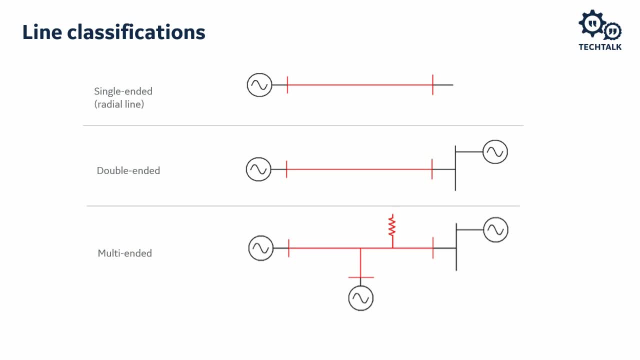 can have a source of fault current. Usually, this type of line delivers power from the source to a load at the other end of the line. Therefore, when a fault occurs, it delivers power in different directions at different times. If a fault occurs on this, 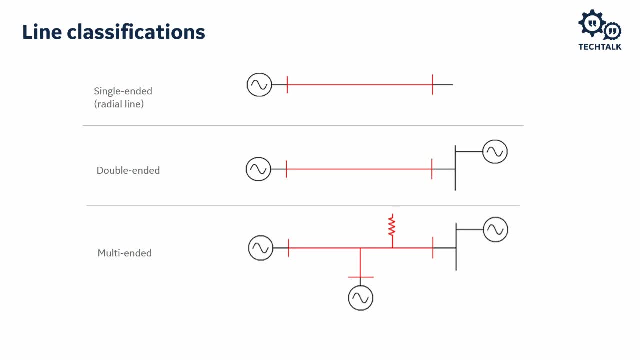 transmission line, current is fed to the fault from two locations. A multi-ended line has more than two boundaries, each of which can have a source of fault: current. For this type of line, the normal power flow varies and at the time of a transmission line fault, the fault is fed. 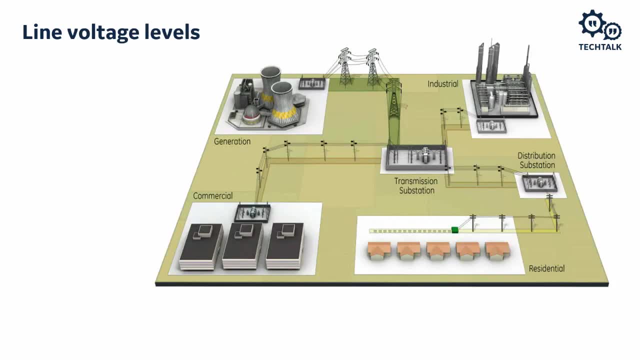 from many different locations. Another way to classify lines is by the voltage level. The voltages that are used for power transmission are split into three categories. Distribution levels are in the range of 2 to 35 kV. Sub-transmission levels are 30 to 150 kV. Transmission levels. 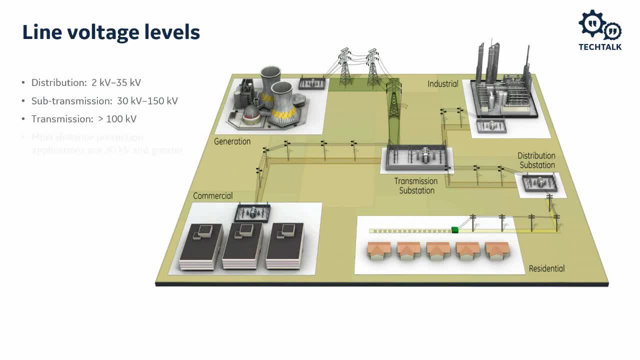 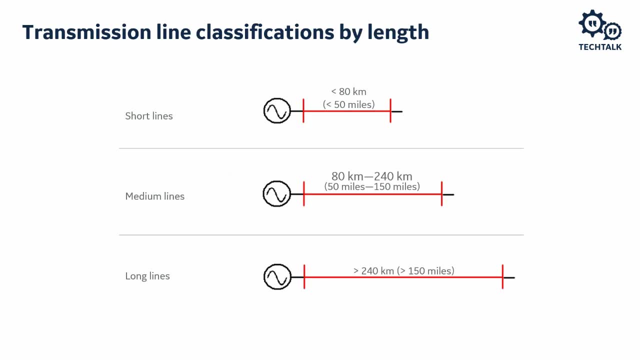 are greater than 100 kV. Most applications that use distance protection are 30 kV and greater. An additional classification for lines is the line length. Short transmission lines are less than 80 kilometers. 50 miles in length. Medium transmission. 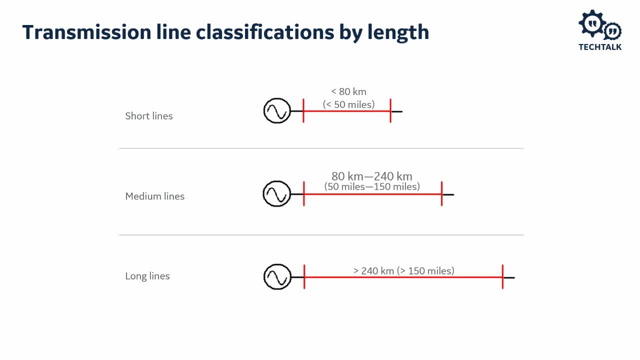 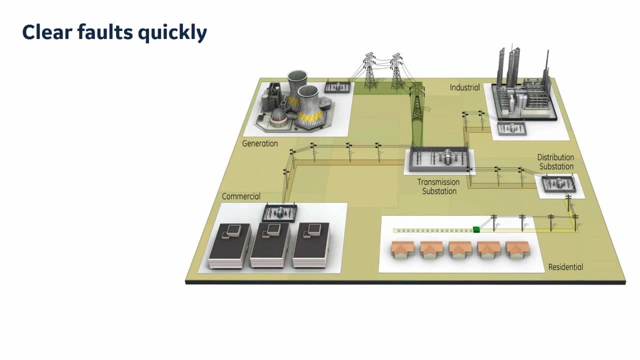 lines are roughly between 80 to 240 kilometers, that's 50 to 150 miles, And long transmission lines are greater than 240 kilometers- 150 miles, in length. Our task is to clear faults quickly. The longer that the fault remains on the line, the greater is the possibility that. 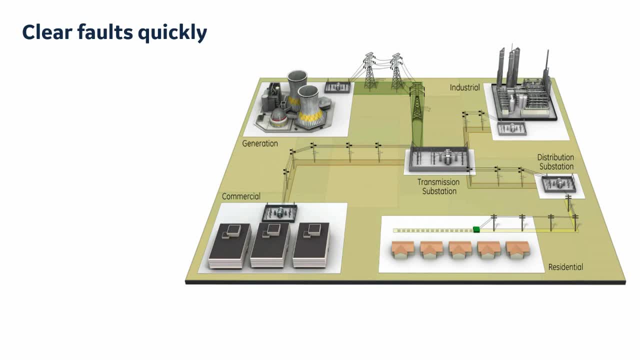 the system becomes unstable and possibly collapses. The engineer's job is to calculate system impedance ratio, SIR, to construct line models like Miller equivalents and to configure accurate settings for the distance relays. Once commissioned, the relay job is to calculate the current at the time of the fault and then to clear the fault quickly. 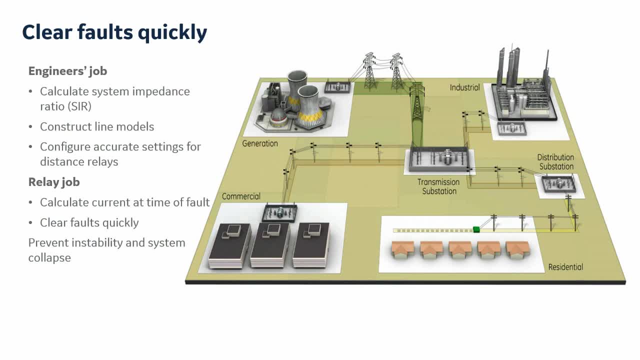 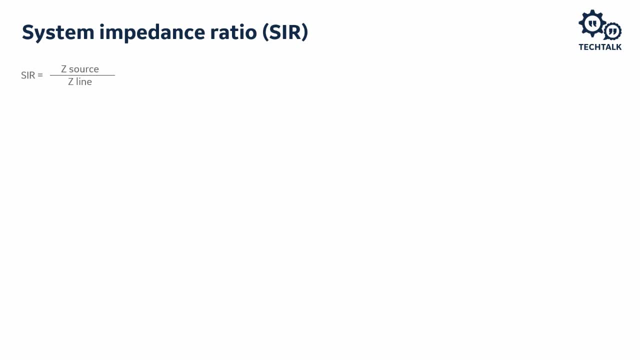 The eventual purpose of these tasks is to prevent instability. So let's look at our first job: calculating the SIR, the system impedance ratio. The SIR takes the source impedance of the system behind the transmission line and divides that by the protected line impedance, So we have Z source over Z line. 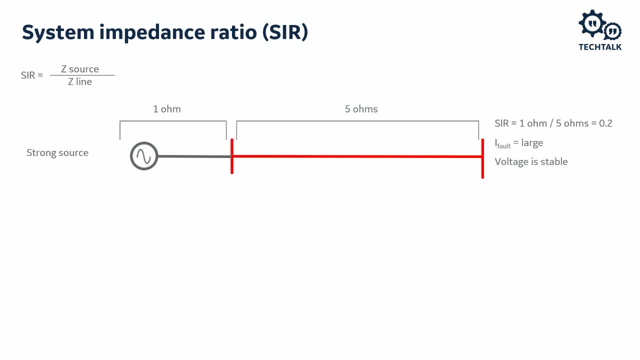 Our first example is a strong source. It has a small impedance of 1 ohm, meaning that this line impedance can provide a LOT of power. If the line impedance is 5 ohms, then the SIR is 0.2.. For this strong source, the fault. 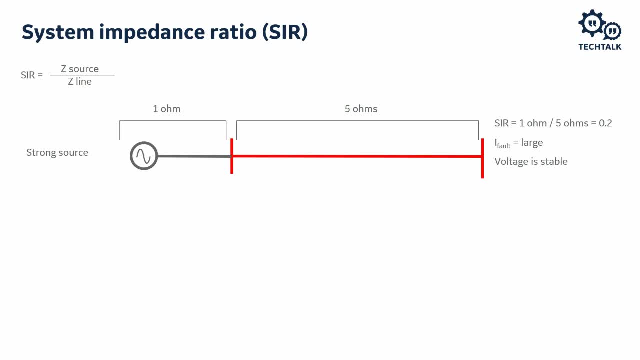 current can be very large and during a fault the voltage remains stable. If the system behind the transmission line is a weak source, then the source impedance ratio is larger. In this example, the weak source has a large impedance of 20 ohms. so 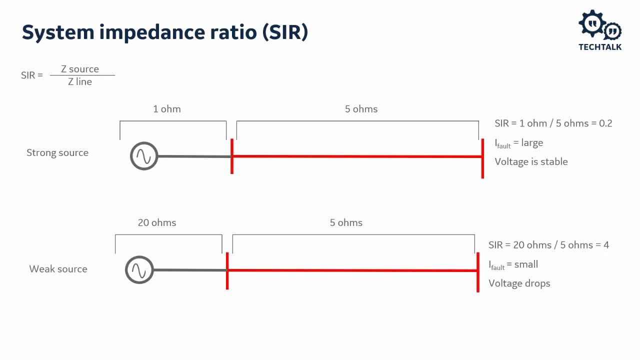 resulting SIR is 4.. When a fault occurs on this transmission line, the fault current is small and the line voltage drops or dips. Therefore, the system impedance ratio is a very important factor in power system stability at the time of a fault. We must consider SIR when determining the type of protection. 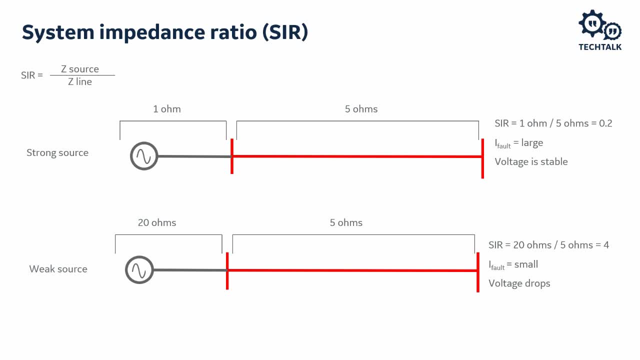 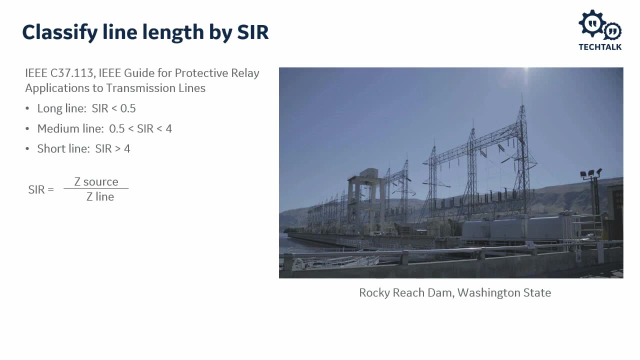 needed and the fault clearing speed needed to keep the system stable. There is another way to classify line length, as specified in IEEE C37.113, The IEEE guide for protective relay applications to transmission lines. Transmission line length is based upon SIR. Longer lines have greater impedance. 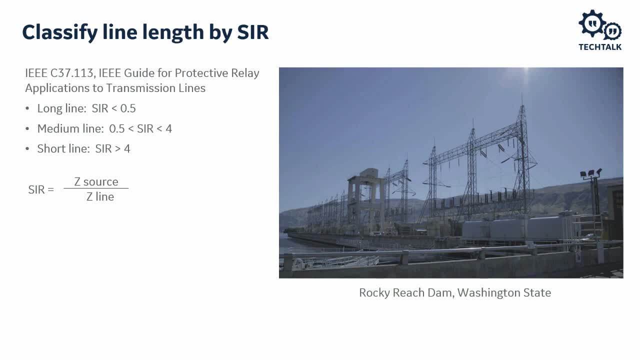 making the SIR denominator larger. Line classifications are these: a long line is SIR less than zero point five. a medium line has SIR between zero point five and four. merely Just click on SIR annotation to narrow it down down 5 and 4. and a short line has SIR of greater than 4.. An example of long lines are those that transmit. 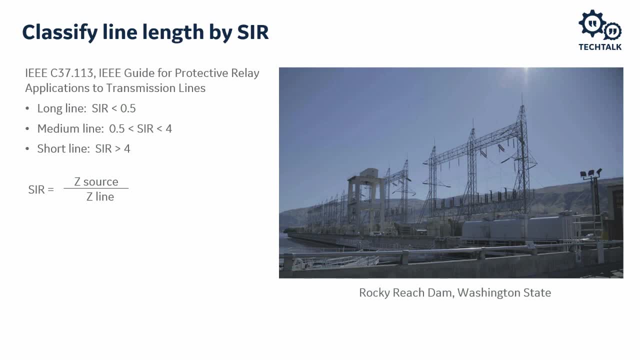 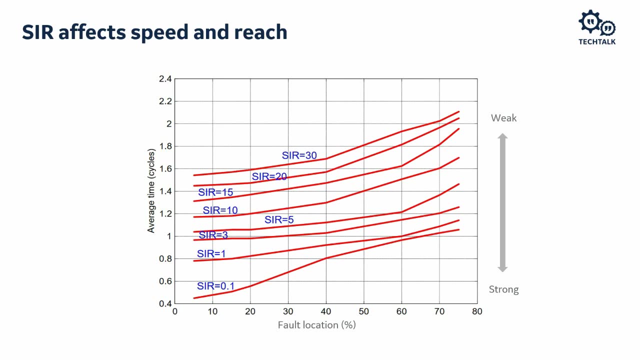 power from hydro facilities. On the screen is a picture of Rocky Reach Dam near my home in Washington state. SIR affects the speed and reach of the distance relay. as you can see from this chart of fault location versus average operate time, Fault clearing speed is slower for large SIRs. 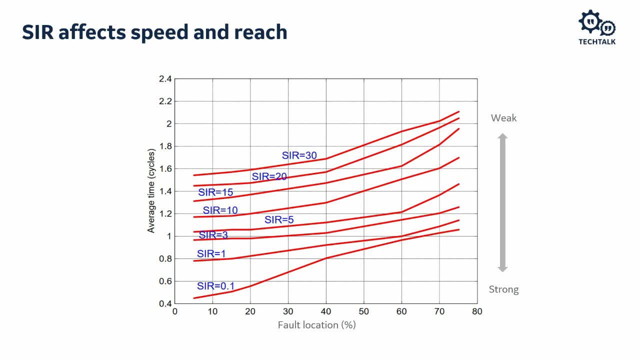 This is because the relay measures smaller voltages and currents. therefore it takes more time for the relay to ensure a secure trip decision. Under reach is a problem as seen here in the tip up on lines with large SIRs. For short lines with SIR greater than 4, you 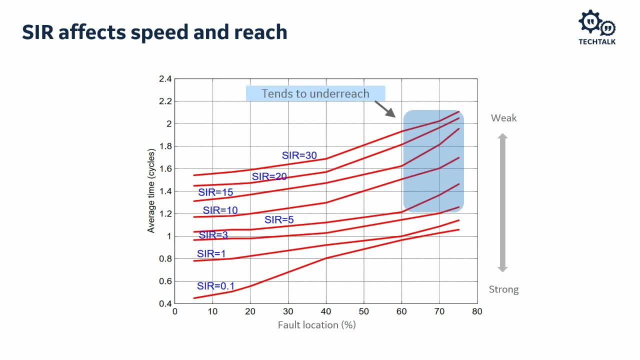 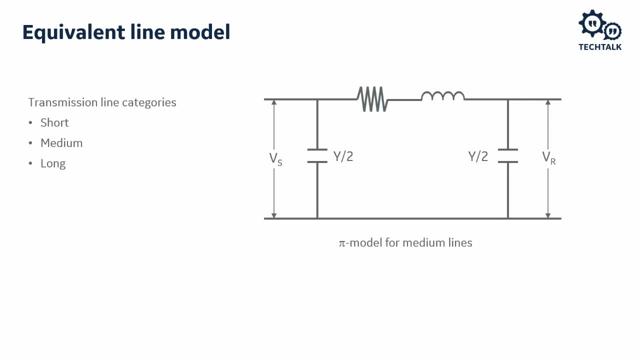 might want to consider other types of line protection, particularly line differential with distance backup. Another job for the engineer is to develop an equivalent line model. These models vary with the line length Over the years. protection engineers have used the PI model shown here to represent medium length lines for hand calculation, Today computer-aided. 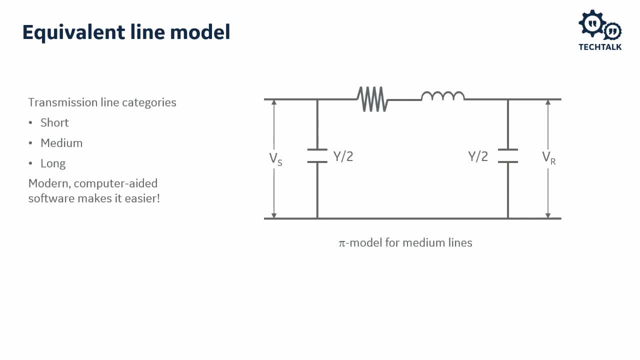 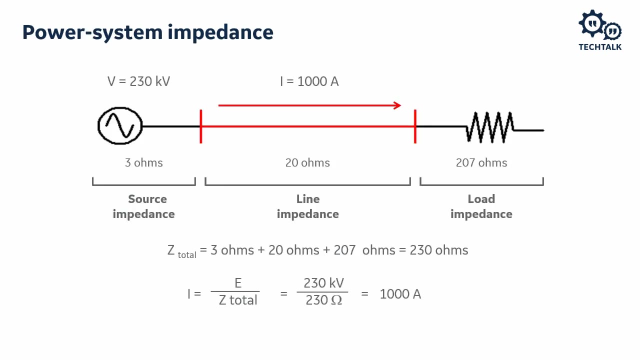 software helps us calculate all required values. The next part of the engineer's job is to configure accurate settings. While software helps immensely, it is important to understand how power system impedance works. Each component in a power system has an impedance. In this system, the total impedance is 230 ohms. 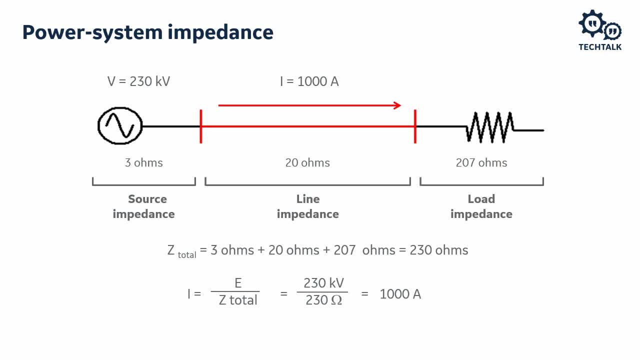 If this is a 400 kV line-to-line system, then the phase to neutral voltage is 230 kV. Ohm's law tells us that 1000 amps of current is supplied to the load. A fault changes the impedance. If a fault 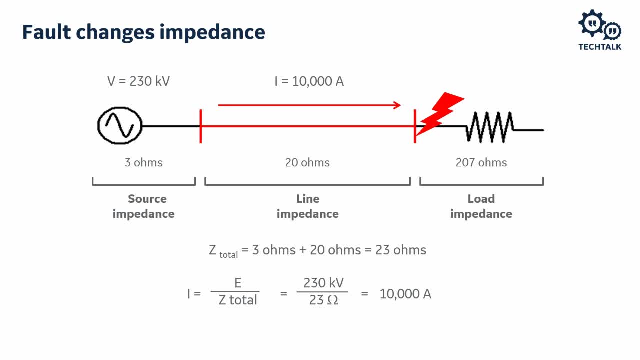 occurs at the end bus, it cuts the power. If a fault occurs at the end bus, it cuts the power. If a fault occurs at the end bus, it cuts the point. If a fault occurs at the end bus, it cuts the current flow, The output level of current increases. The blue piece represents the 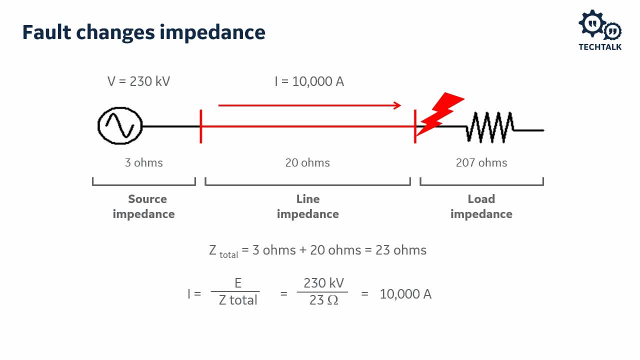 total impedance of the current flow, Then the total impedance of the power system changes to only 23 ohms. This drop in impedance increases the current level substantially. A relay at the left side bus would measure 10,000 amps of fault current. 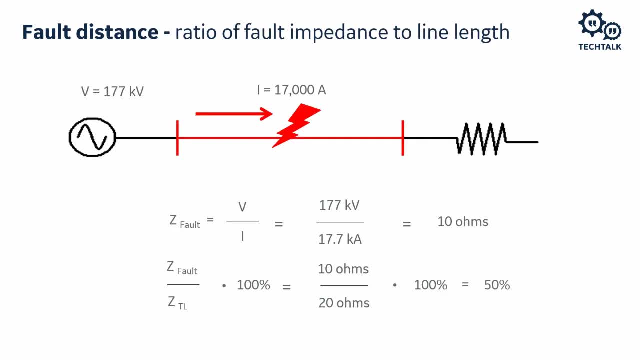 The relay uses the measured voltage and fault current to determine the fault distance along the line. Suppose that the fault is in the middle of the protected line. In this example, we have a weak source and so the voltage drops to 177 kV from the 230 kV line to neutral voltage. 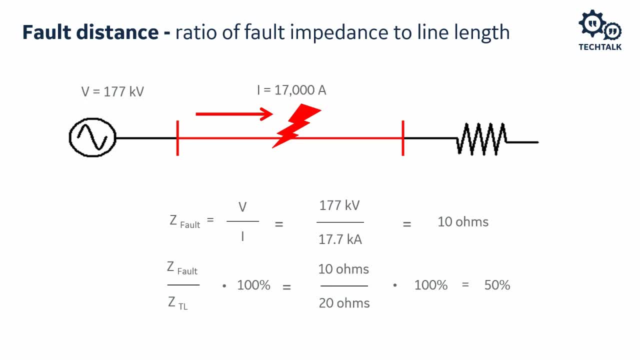 The distance relay measures this reduced voltage and the substantially larger current of 17,000 amps. Now the relay determines a faulted impedance of 10 ohms, which is half of the 20 ohm total line impedance. It declares a distance of 50% down the transmission line. This is where we get the term. 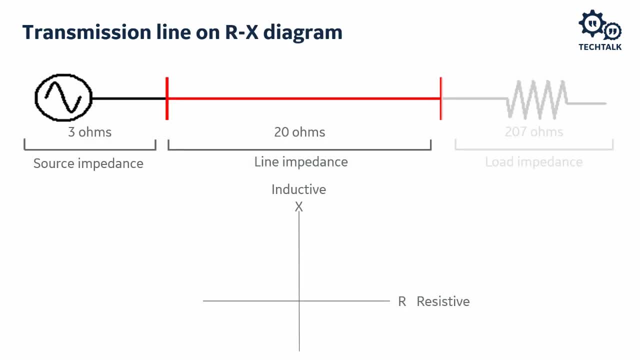 distance protection. Let's take a closer look at our 20 ohm transmission line. on an Rx diagram, The horizontal x-axis represents the resistive component of the impedance of the line. The vertical y-axis represents the inductive component of the line impedance. 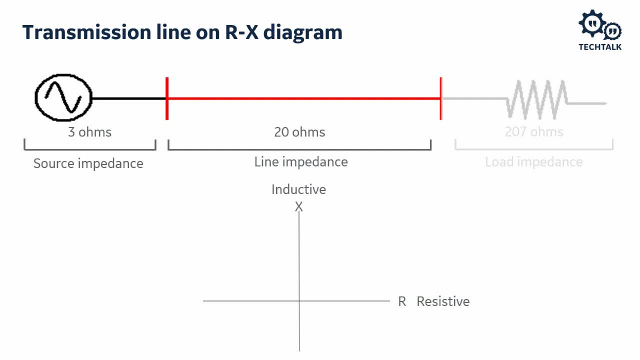 Although the sign for inductive reactants in electronics is negative, in the distance protection world we consider inductive as up or positive, so we don't have to write so many negative signs. The impedance of a transmission line is mostly inductive. Therefore, when we plot the impedance of the line it is very close to the y-axis. 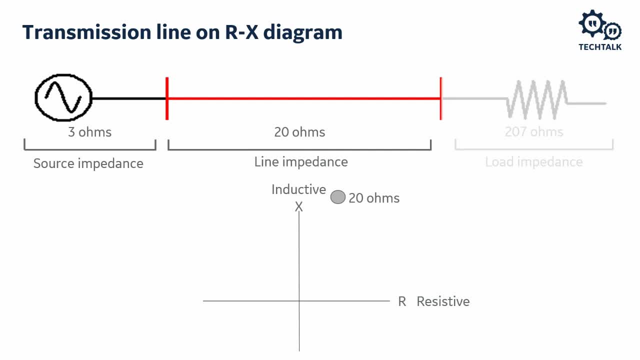 as shown here on the 20 ohm point. If a line is drawn from this impedance point to the origin, we have a representation of the entire transmission line. For example, you can plot the 10 ohm midpoint of the line as shown. 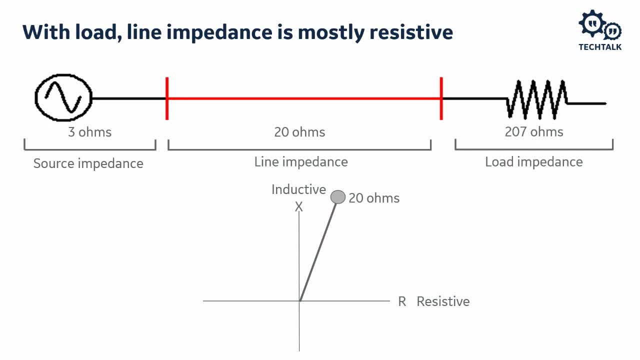 With load, the measured impedance is mostly resistive. In a normal power system there is a load at the end of the transmission line. Typically this load is resistive and is larger than all other power system impedances. Therefore, when we plot the power system impedance under normal conditions, 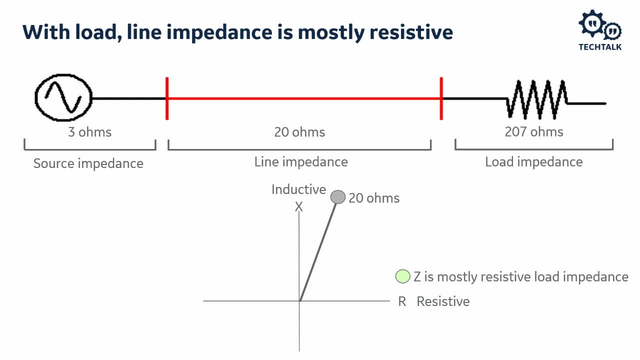 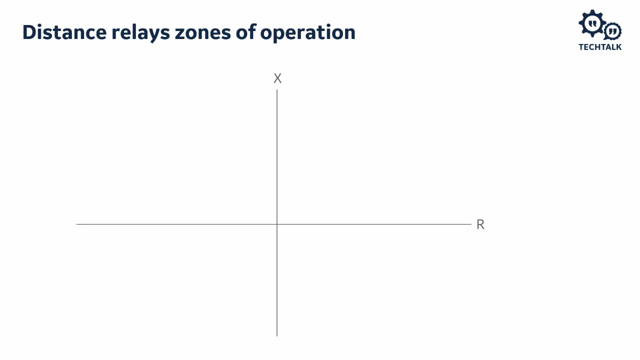 the measured load point is very close to the x-axis. With a fault, the measured impedance is mostly inductive and the load loses power. Now let's explore distance element zones of operation. Modern distance elements operate according to zones on the Rx diagram. If the relay calculates: 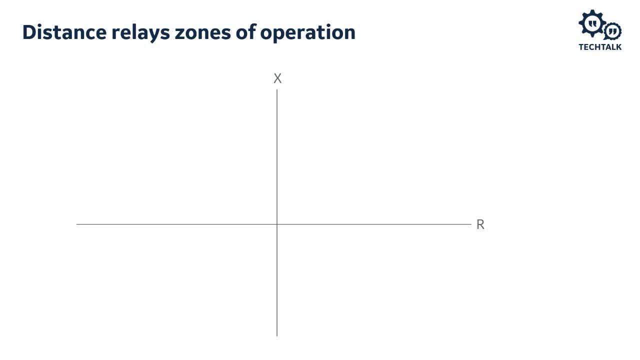 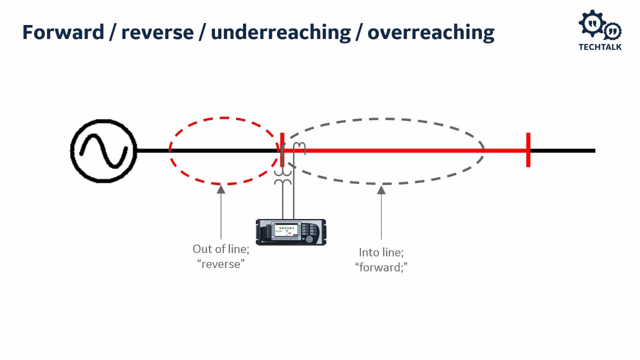 power system impedance within a zone, then the relay trips. The operation zones are these: The impedance zone, the admittance or MO circle- mostly inductive reactance- the reactance zone, the resistance zone and the quadrilateral zone. Zones can be programmed to protect in either the 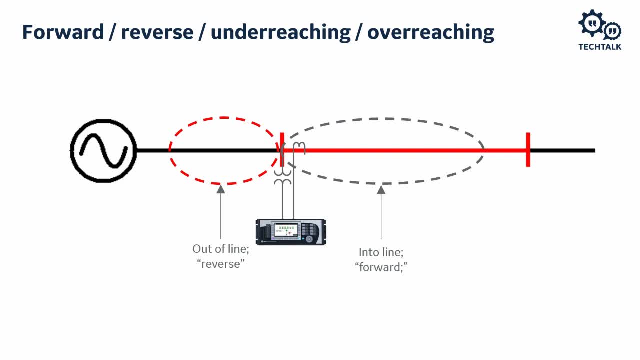 forward direction or in the reverse direction. We say into the line when zones are set to protect in the forward direction. We say out of the line when zones protect in the reverse direction. Shown here is an under-reaching zone on the forward line. If the zone extends past the 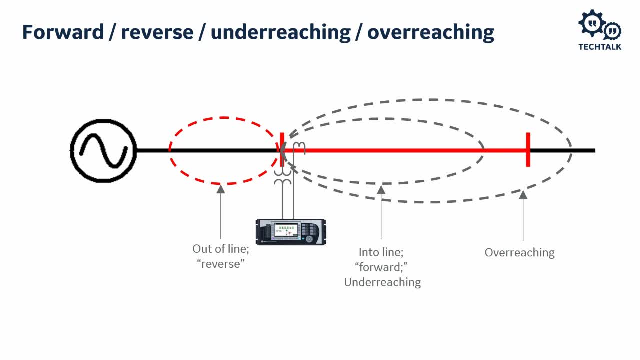 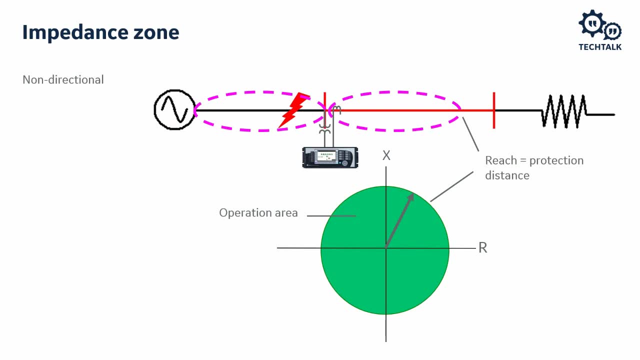 protected line, then the resistance zone is protected. If the resistance zone extends, then it is an over-reaching zone. This is an impedance zone. Any impedance that falls within the radius of the circle indicates a fault. Note that the reach is the distance along a portion of. 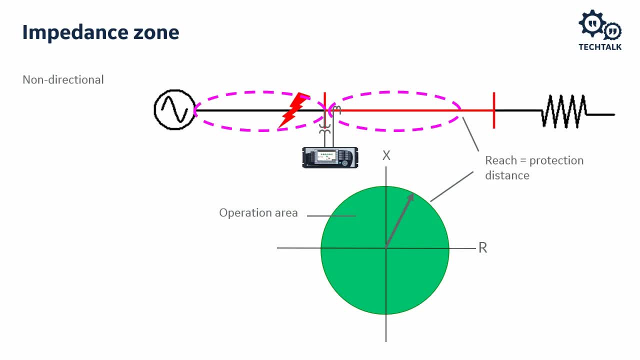 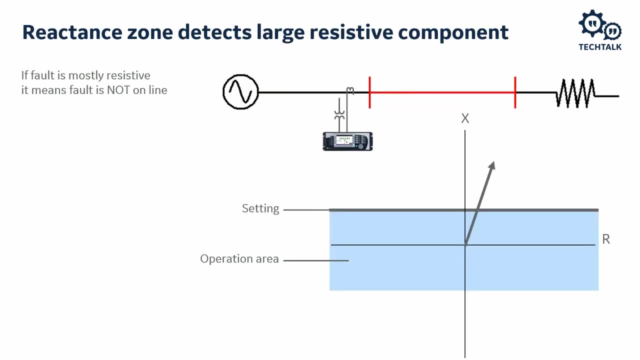 the protected line, which is in the protection zone. An impedance zone is inherently non-directional and detects faults that occur in the reverse direction away from the point of measurement. This type of impedance zone is normally used for generator backup protection. The zone of operation shown here is a reactance zone. This zone detects when the impedance of the 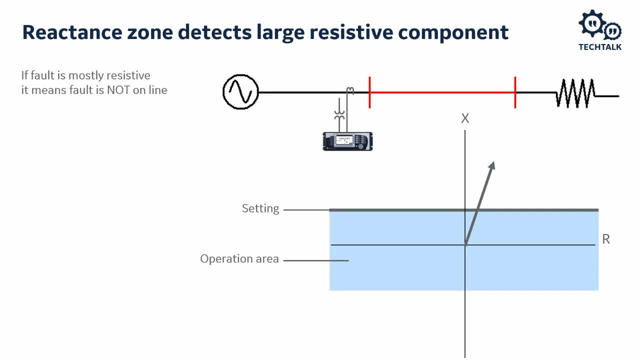 fault has a very large resistive component. It indicates that there is load on the system. If there is a fault, then that fault is not on the transmission line. Usually, this type of zone is not used to trip a transmission line on its own. Instead, it is used to supervise another. 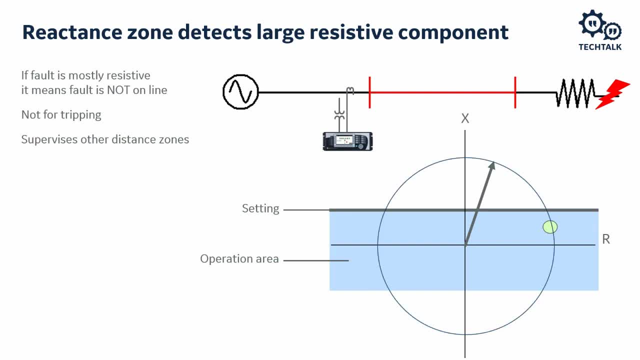 distance zone of protection. For example, if a relay detects that an impedance enters the impedance zone because of an external fault, the reactance zone blocks. It determines that the impedance is mostly resistive and does not trip. Therefore the fault is not on the 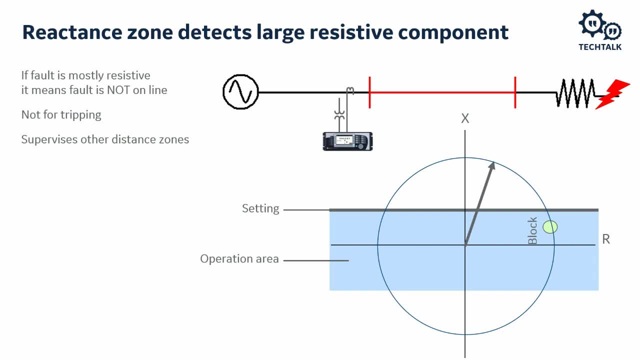 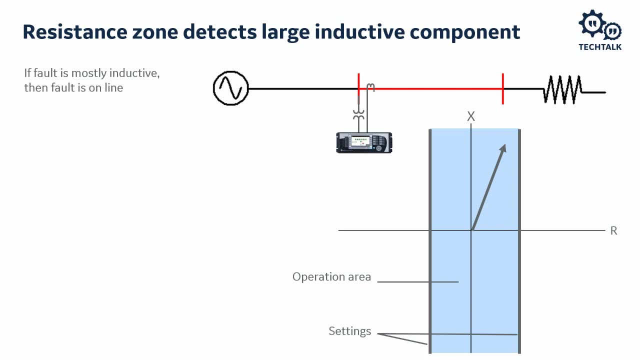 transmission line- Remember this word- blocks. The zone of operation shown here is a resistance zone. This zone detects when the impedance of the fault has a very large inductive component. If the fault does have a large inductive impedance, this indicates there is very little. 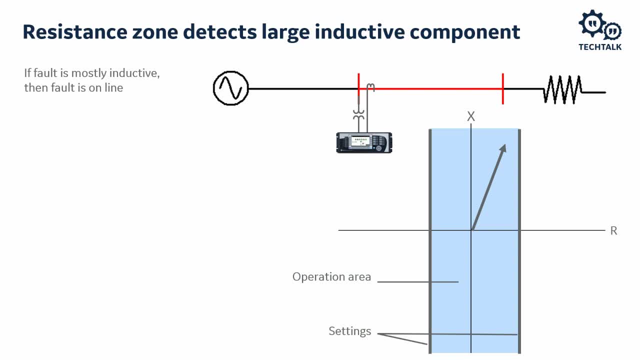 or no resistive load at the end of the transmission line, So it's likely that the fault is located on the transmission line itself. The set points, the two lines crossing the x-axis don't have to be the same. Usually this operational zone is not used to trip a transmission line on. 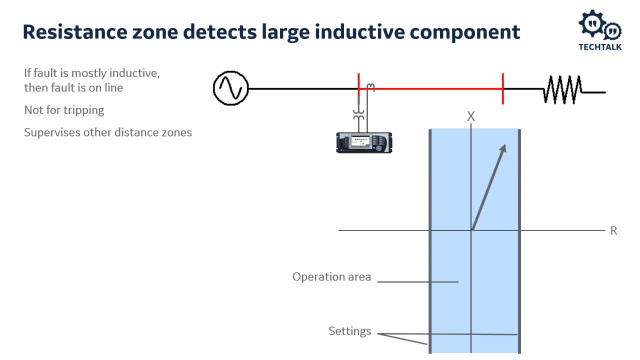 its own. Normally it supervises another distance zone. For example, for a fault towards the end of the line, the relay detects that an impedance has entered its impedance zone of protection. The resistive zone verifies that the fault is actually on the transmission line, because the 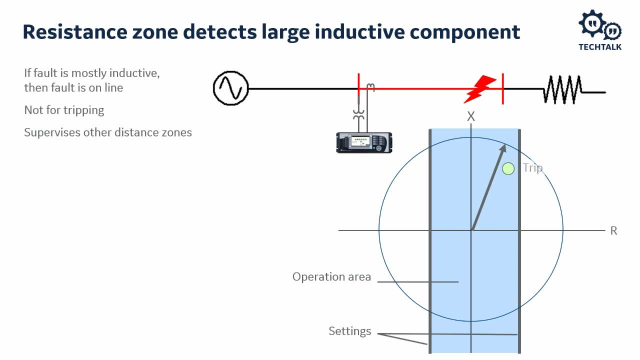 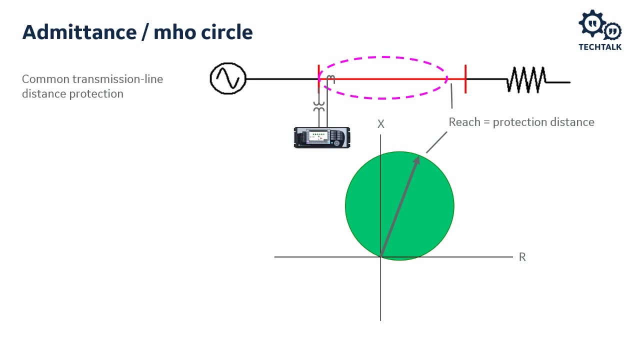 impedance of the fault is mostly inductive. In this configuration, the resistance zone gives the impedance zone permission to trip. Remember this word permission. The protection zone shown here is an admittance zone, what most people call a moh circle, The moh. 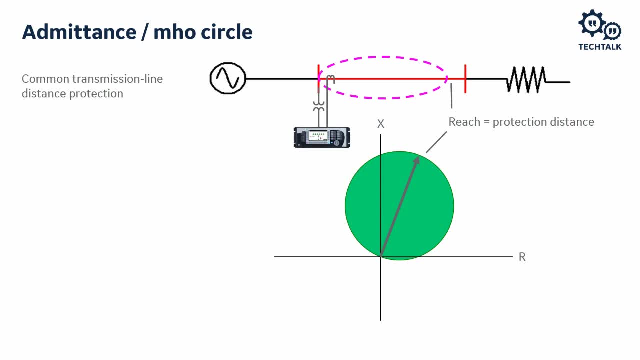 circle zone is the most common type of protection zone used in transmission line distance relays. A moh zone detects when an impedance enters the area defined by the circle. This zone is inherently directional and does not detect a fault in the reverse direction of the transmission line. 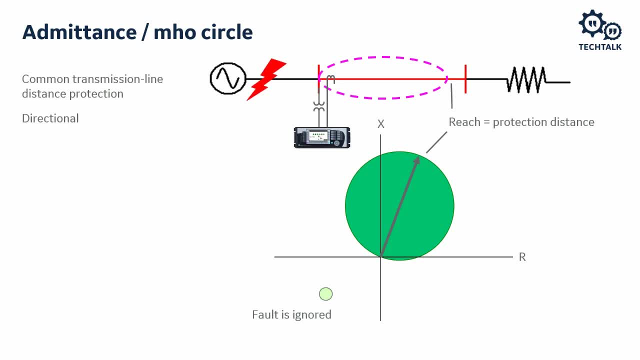 A reverse fault falls outside of the circle, as shown here. We call this circle the self-polarized moh because the relay uses the faulted phase voltage and memory for polarization. Polarization assists the relay to compute impedance. Sometimes we use non-faulted voltages for polarization. I'll have more on this later. 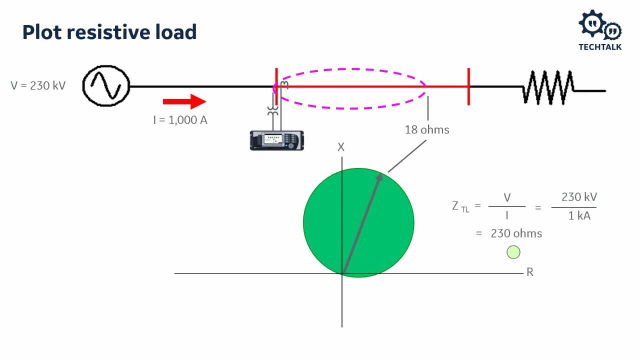 We can plot resistive load on the Rx plane along with the moh circle. Here. the relay measures 1000 amps with 230 kV line to neutral voltage. The impedance locus of this load is 230 ohms. If we add a substantial amount of load, the current needed to feed the load increases. 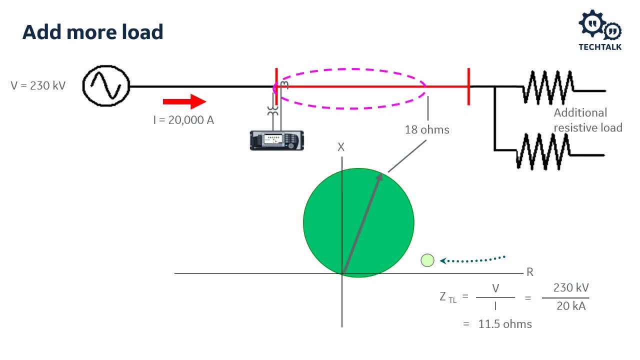 substantially, as seen here. The current needed to feed the load increases substantially, as seen here. Although there is no fault on the transmission line, the newly calculated impedance of the line is less than the overall reach of the moh zone. However, because the added load is mostly 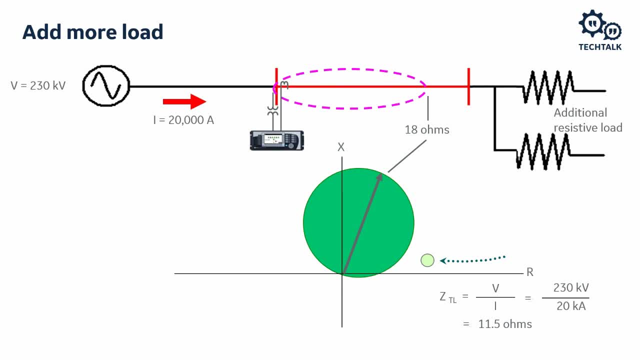 resistive. the plotted impedance point moves toward the graph origin very close to the x-axis, as seen here. Because the moh zone is positioned where it is on the graph, there is very little area included in the x-axis resistance direction. Therefore, the new impedance 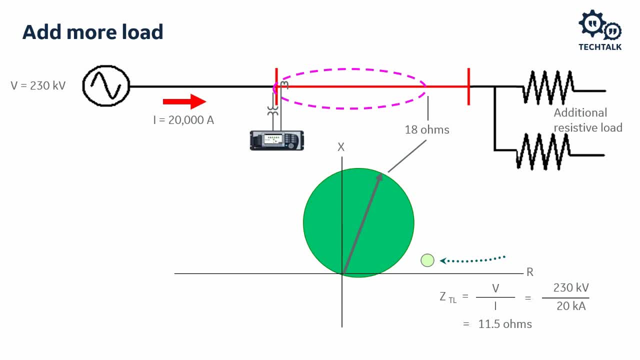 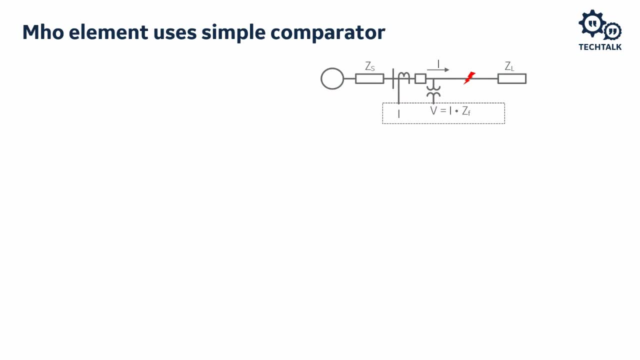 does not fall into the moh zone of protection and the relay does not trip. How does the relay compute the moh characteristic? It uses comparators. Recall that the moh function uses the current and voltage measured at the relay shown in the dashed line box to determine if the apparent impedance falls within the moh. 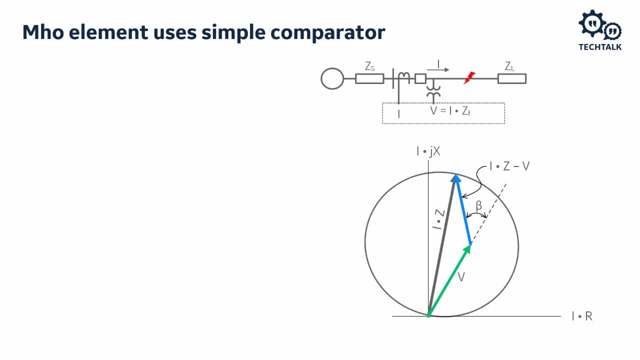 characteristic. A simple moh distance function with a reach of z ohms is shown here in a voltage diagram. This voltage diagram is exactly equal to an r-x diagram, except that all of the impedance vectors have been multiplied by the current i. As before, the total line voltage is i times z. The relay develops two voltages. 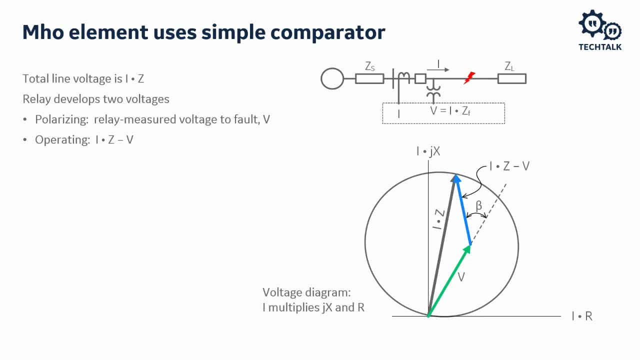 the polarizing voltage v, which is the measured fault voltage, the green phasor and the operating voltage, the difference between the total line voltage and the polarizing voltage i times z minus v. the blue phasor. Plotting these phasors we create the supplementary angle beta. 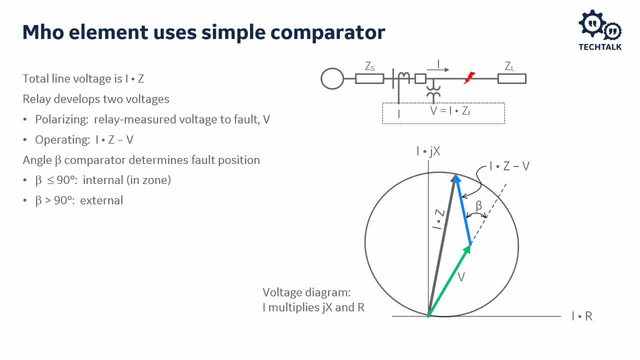 The relay compares this beta angle to 90 degrees. If the result is less than or equal to 90 degrees, then the fault impedance zf, plots within the moh characteristic and the function produces an output. If the result is greater than 90 degrees, then zf falls outside the characteristic. 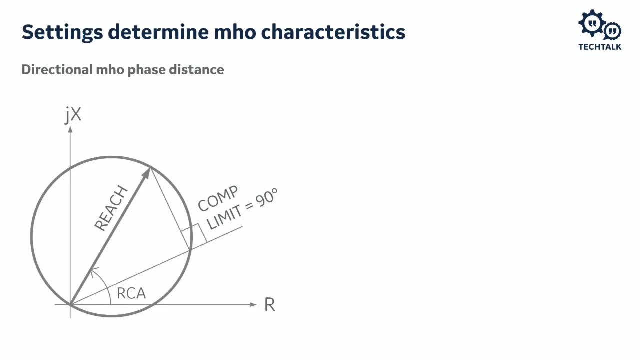 and the fault is out of the zone. Relays have settings to model the moh characteristic along the transmission line. The primary setting is reach, a line impedance magnitude that determines the radius of the circle. The angle at which to place the reach is the RCA reach characteristic angle. 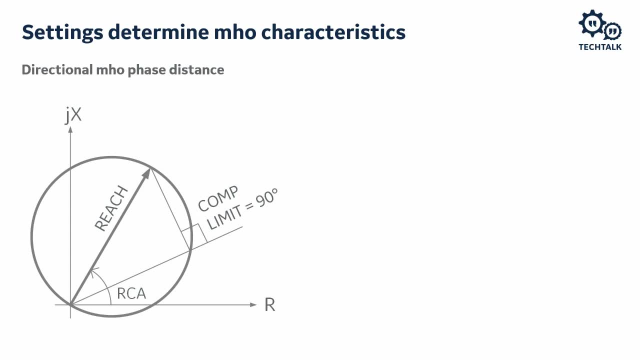 This is the line impedance angle, formerly known in electromechanical relays as the maximum torque angle, MTA. There are no moving parts to develop torque in a micropressor. The setting can limit the comparator angle which makes the moh circle into a lens. 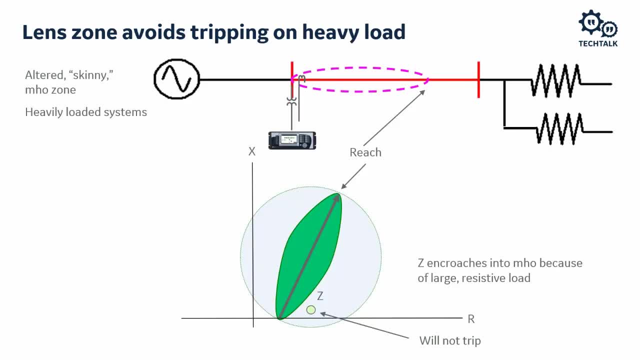 shown here on the right. An advantage of the lens is that it removes much of the resistive coverage of the moh circle. If this power system is heavily loaded then this load impedance might encroach into a normal moh circle. The lens zone avoids tripping on heavy load. 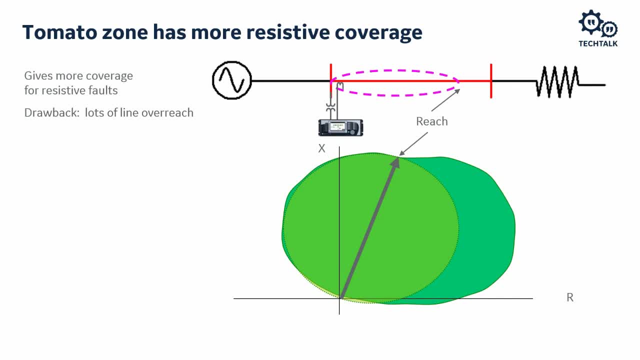 Another alteration of the moh circle is a tomato shape. It detects faults that have a resistive nature, giving coverage along the x-axis. A major drawback is that there is significant line overreach. In a moment we will see how a quadrilateral shape gives resistive coverage without line overreach. 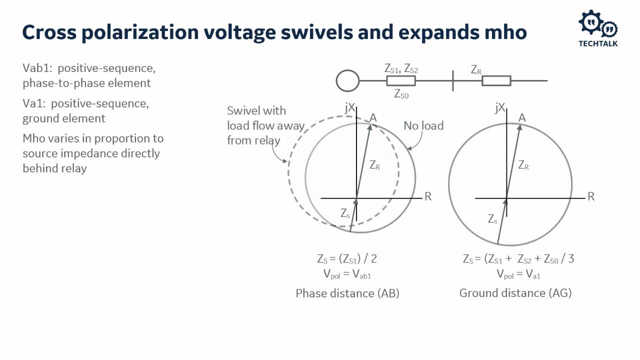 Another method to accommodate more fault resistance is cross polarization. This is when we set the relay to use other than the faulted voltage. This is a big topic and I am not going to discuss all types of cross polarization in this presentation. Cross polarization retains the circular characteristic, but the circle can. 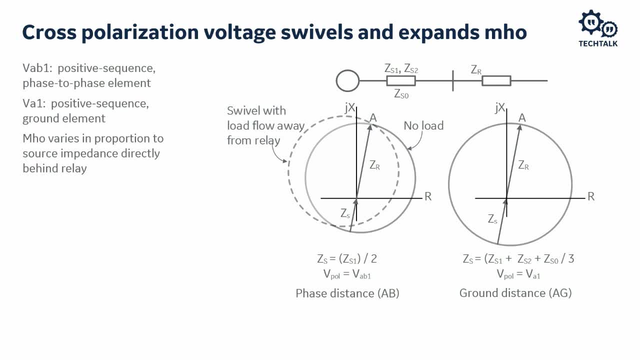 swivel, and it can vary in size depending upon system conditions. For example, consider a distance function that uses positive sequence voltage as the polarizing signal. The characteristics for a phase distance function and a ground distance function with positive sequence voltage polarization are shown here. As can be seen, these characteristics are not fixed in size. 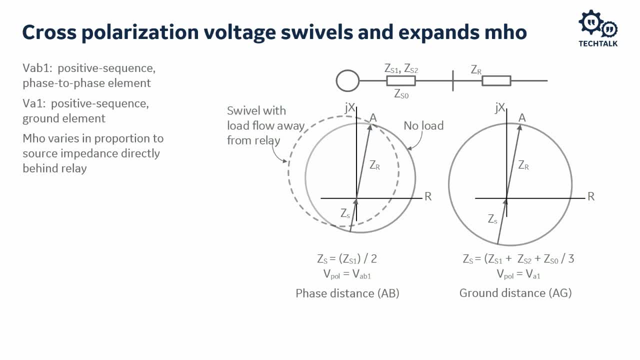 but vary proportionally with the source impedance directly behind the function For the left phase distance diagram, load flow causes the characteristic to swivel to the left, as shown, and to the right relative to the forward reach. point A, The amount and direction. 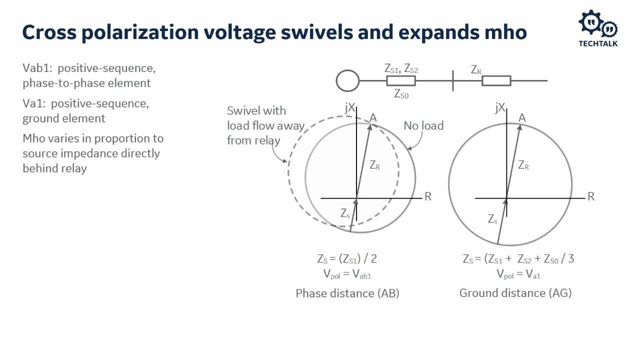 of the swivel depends upon the magnitude and the direction of load flow. For the right ground distance diagram, the characteristic expands proportionate to the source impedance. Again, the effect of the swivel and size variation is to accommodate more resistance in the fault. 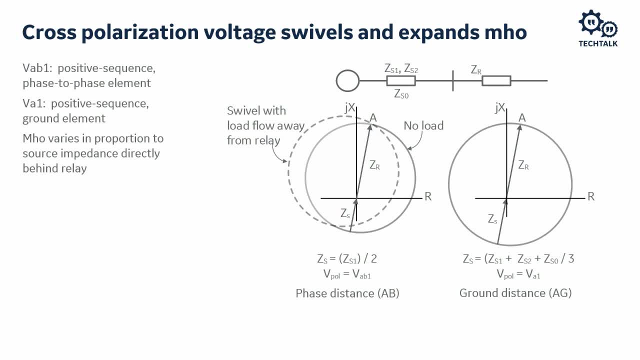 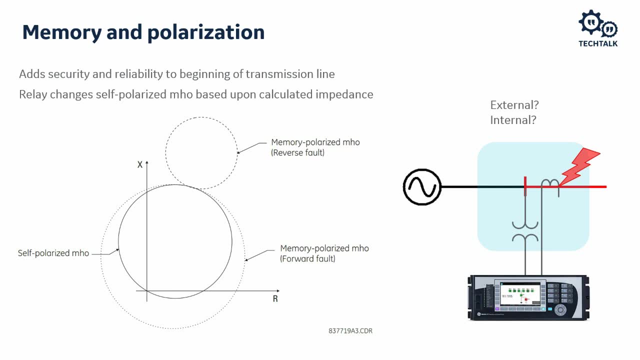 than would be obtained with a self-polarized MOE function. For a fault right at the relay location, the voltage will be very small, approaching zero for a bolted fault, and a self-polarized MOE function might not operate. 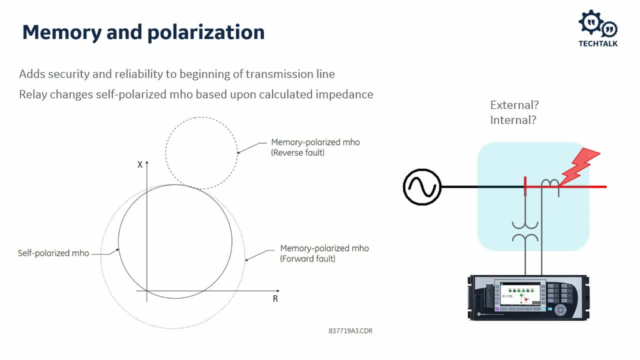 The cross-polarized MOE we just discussed is one solution, except in the case of a three-phase fault. For a close-in three-phase fault, all three voltages will be very small. Therefore, operation of any of the cross-polarized functions is jeopardized. 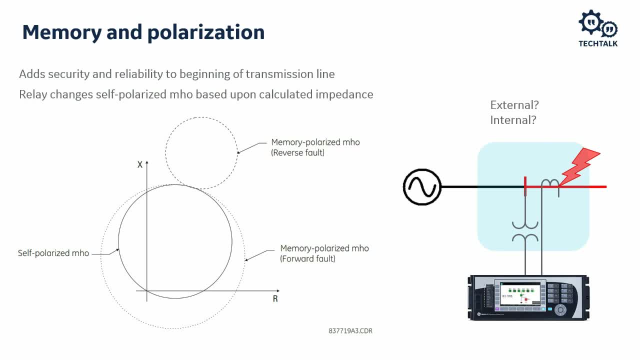 because there will be very little or no voltage available to develop the polarizing quantity. To overcome this problem, the relay uses fault voltage memory for polarization. This adds security and reliability for faults that occur very closely to the relay measurement point shown here, highlighted in blue. 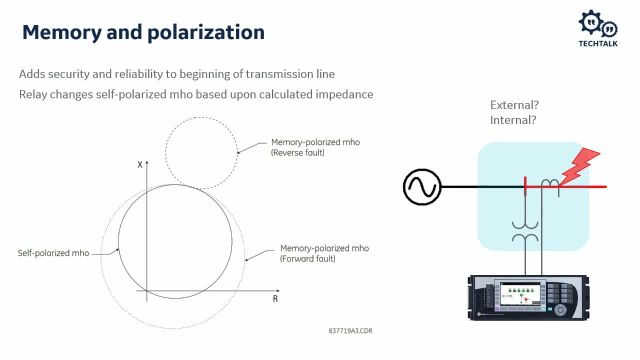 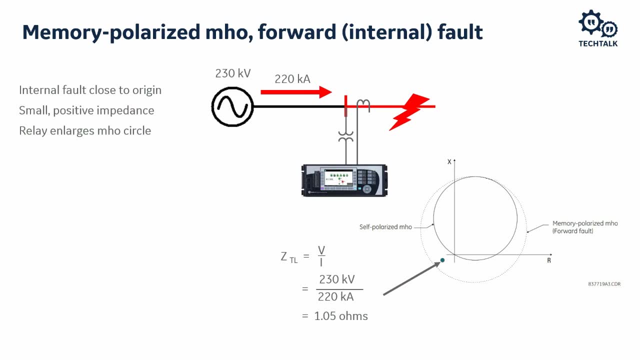 With memory. the relay changes the size of the MOE circle when the calculated impedance is very close to the origin. In this example, a fault occurs just after the beginning of the transmission line. Current flows into the CT from the positive direction. The relay calculates the impedance of the line as positive. 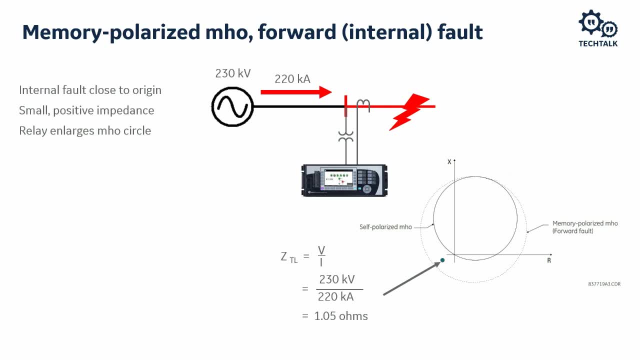 This impedance point plots very close to the origin and in the positive direction of the line. The relay recognizes this small positive line impedance and enlarges the radius of the circle. It trips for this fault properly. Notice that the reach of the MOE circle did not change. 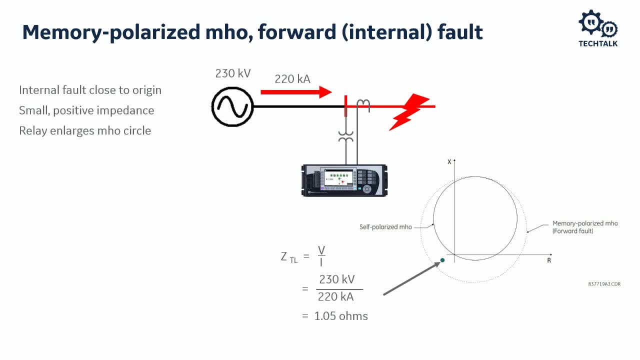 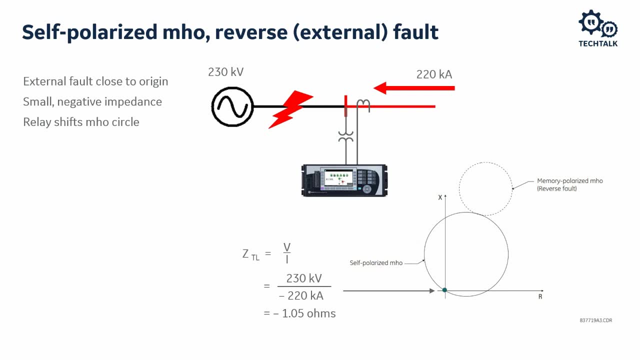 and still extends out to the end of the original zone of protection. In this example, a fault occurs just before the beginning of the transmission line and current flows into the CT from the opposite direction. Now the relay recognizes this small positive line impedance. 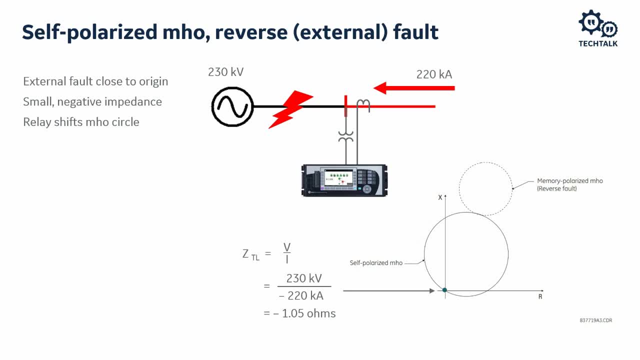 and shifts the circle, The relay calculates the impedance of the line as negative. This impedance plots in the reverse direction, very close to the origin. To ensure that the MOE characteristic does not interpret the impedance as an internal fault, the relay recognizes the small negative line impedance. 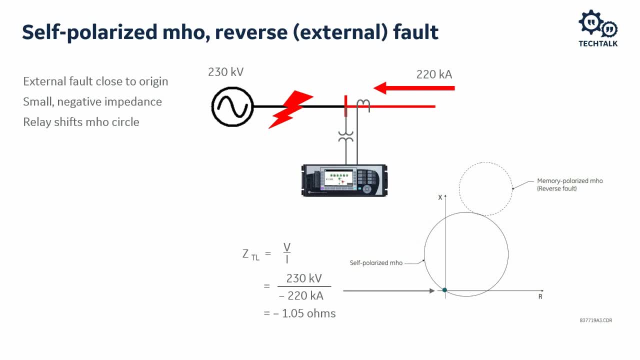 and shifts the circle. Because the new MOE circle is not near the fault location next to the origin, there is no chance of the relay false-tripping. Notice that the reach of the Mohr circle does not change and still extends out to the end of the original zone of protection. 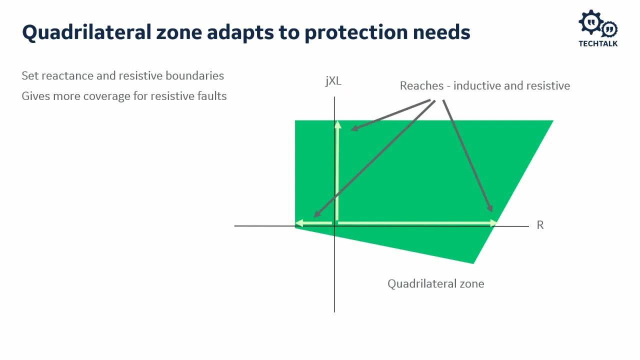 Another way to increase fault resistance coverage is the quadrilateral zone characteristic. A modern relay has the calculation power to create a quad zone of protection from the measured voltages and currents. For the quad there are essentially two reaches: one in the inductive direction and one in the resistive direction. 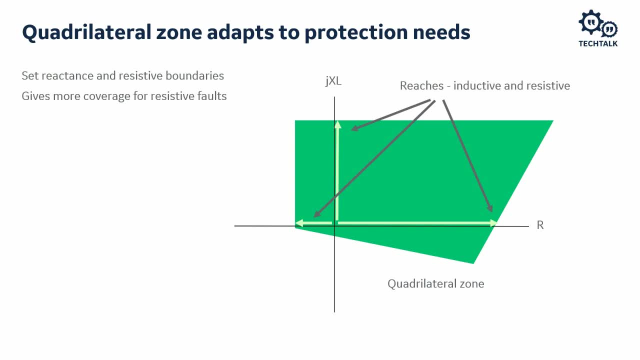 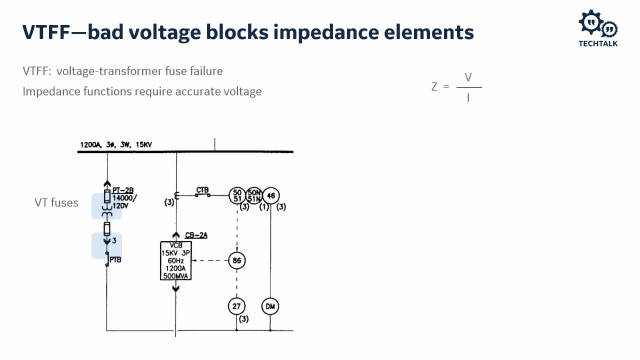 Set the reactants and resistive upper and lower boundaries to create a custom shape to match the needs of your power system protection. To me these quad characteristics look like old-fashioned military surplus camping tents. Element settings rearrange the tent poles. Voltage is essential to measuring impedance. 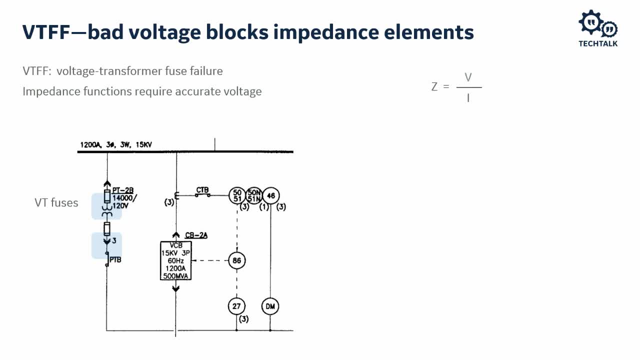 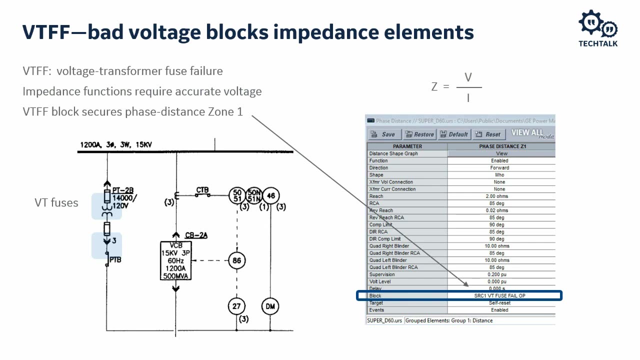 Distance protection relies on valid voltage. Loss of voltage appears as a close-in fault for distance elements. If there is a VT fuse failure or other VT problem then we must block the distance elements to prevent nooses operation. Note that ground distance zone 1 does not require these measures because zero-sequence current, which is not affected by load current, operates the ground distance protection. 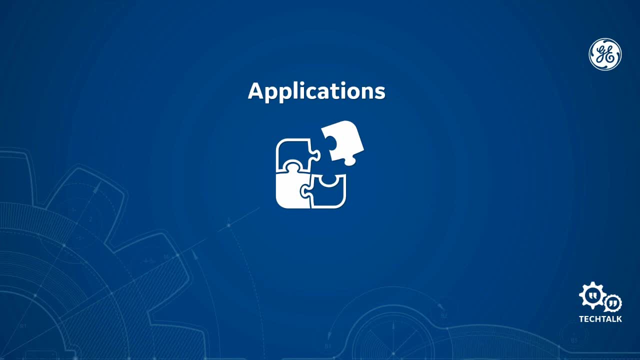 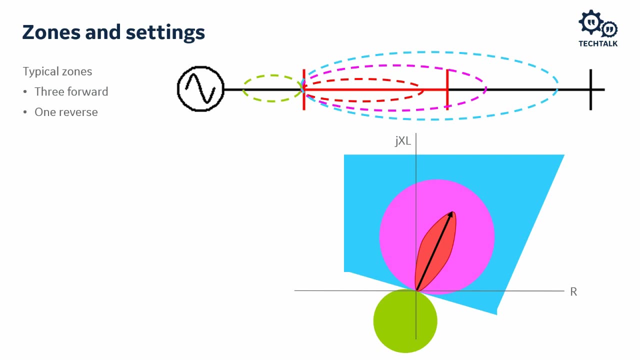 Now that we know how it works, let's take a look at some distance protection applications. A typical application of the distance protection zones is three forward zones and one reverse zone. The zones can be set to have a MOE or quadrilateral shaped protection characteristic. 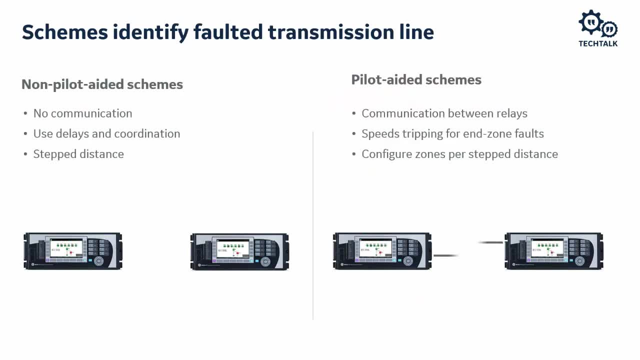 The strategy used to protect a line is called a scheme. All protection schemes used in distance protection fit into one of the following two categories: Non-pilot-aided schemes and pilot-aided schemes. The main difference between the two types of schemes is that in pilot-aided schemes, 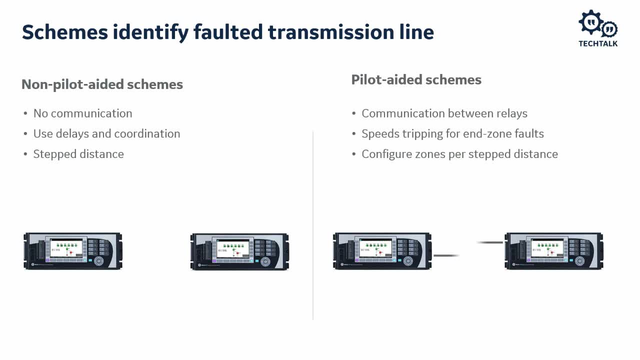 the distance relays communicate with each other to identify whether the fault is located on the transmission line. This speeds line clearing, especially for an end-of-line or end-zone fault. The relays used in non-pilot-aided schemes do not communicate. 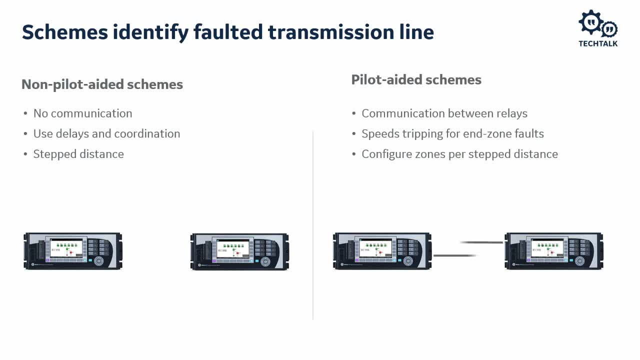 Instead, these schemes use delays and other forms of coordination to determine whether the fault is located on the line. All coordination in these schemes is done within each relay in a stepped distance scheme. It's important to note that the stepped distance scheme is the basic structure for both non-pilot and pilot-aided schemes. 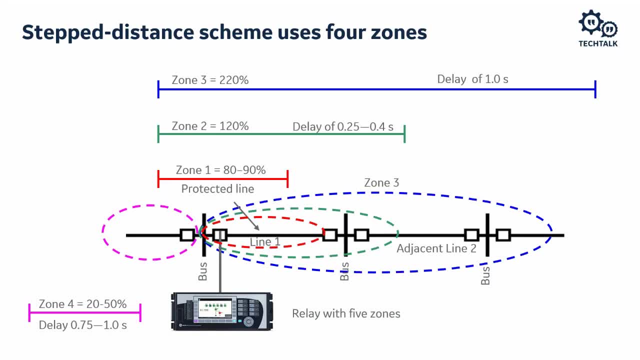 Let's investigate the stepped distance scheme. The relay with a stepped distance scheme uses four different zones to protect its own transmission line and to back up protection on adjacent transmission lines. Zone 1 underreaches the protected line at 80-90%. Setting it any longer leads to false tripping from faults in adjacent line 2.. 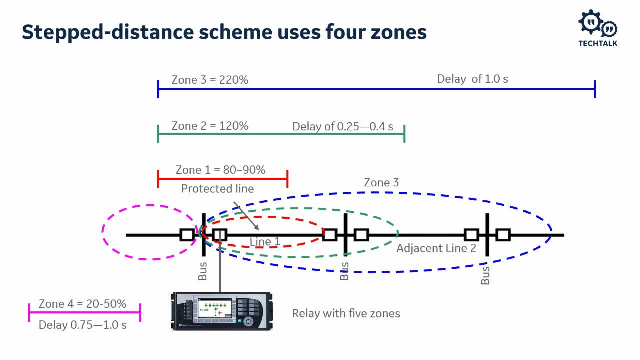 There is no delay in Zone 1.. Zone 2 overreaches the protected line, reaching into the adjacent line. Usually the Zone 2 reach setting is 120%. Other relays have responsibility for the 80% to 100% end zone. 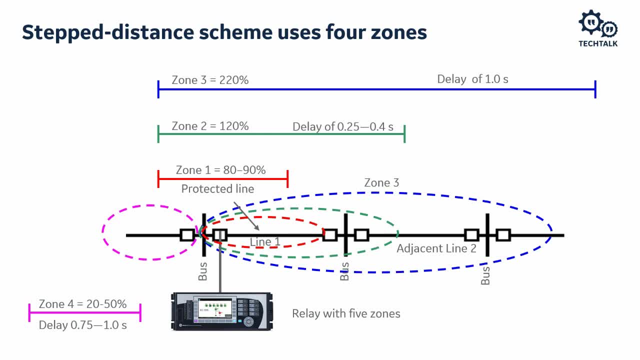 so we set a delay in Zone 2 to let these relays operate first. Zone 3 reaches out to 220%. It is last resort coverage if the Line 1 relay and the Line 2 relay fail to operate. Typically there is a long delay of one second. 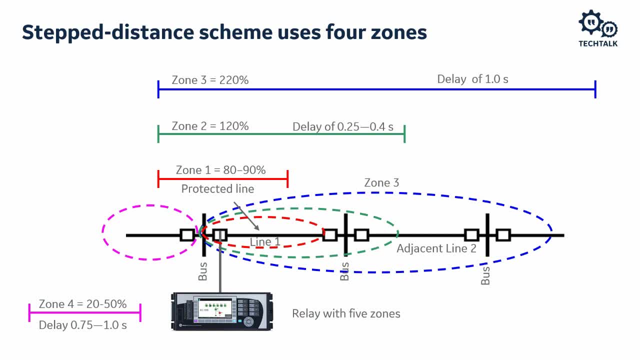 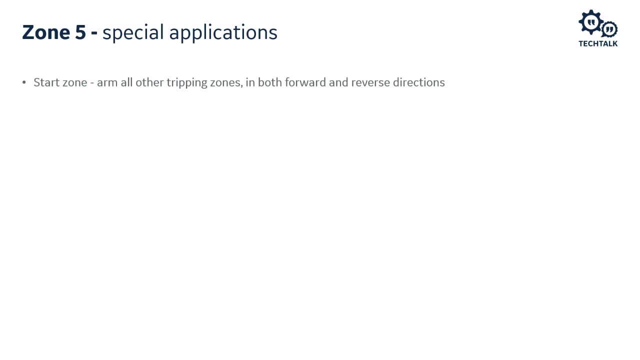 Zone 4 is reverse and covers a section of the reverse adjacent line. if protection for that line fails, There is a long delay of 750 milliseconds to one second for this backup protection. The relay has five zones. Zone 5 is used for various special applications. 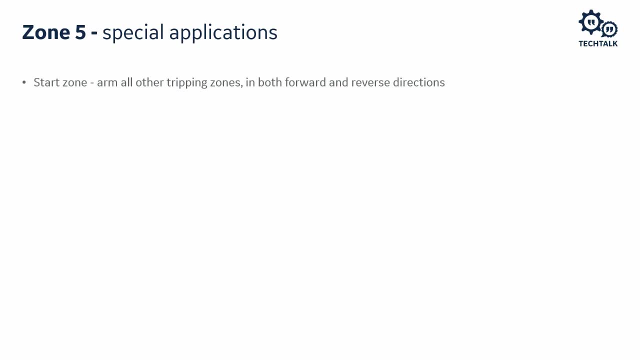 As a start zone for arming all the other tripping zones in both forward and reverse directions As an additional backup protection for reverse. And Zone 5 can be used as an alarm zone for indicating that the load impedance is approaching zone characteristics. These days, most distance protection has communications aided. 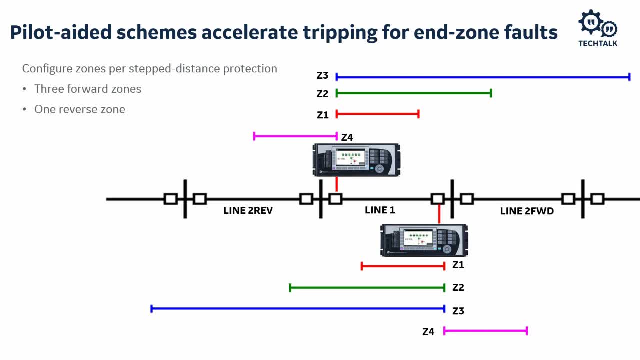 or pilot aided schemes. We configure pilot aided schemes based upon stepped distance protection with three forward zones and one reverse zone for the two relays that protect a line. The relay on the left is the local relay and the relay on the right is the remote relay. 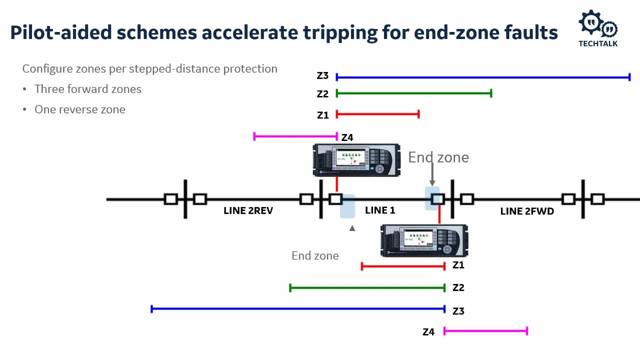 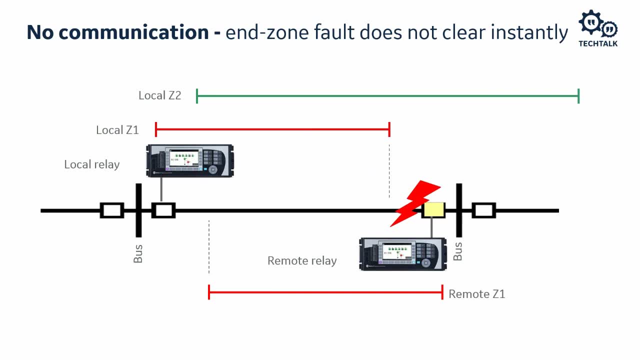 In stepped distance scheme with an underreaching Zone 1 we have an end zone where tripping is delayed. Here two relays are configured with the communications channel in between. If the fault is located in the end zone of the local relay, then the local relay cannot trip the line for this fault instantly. 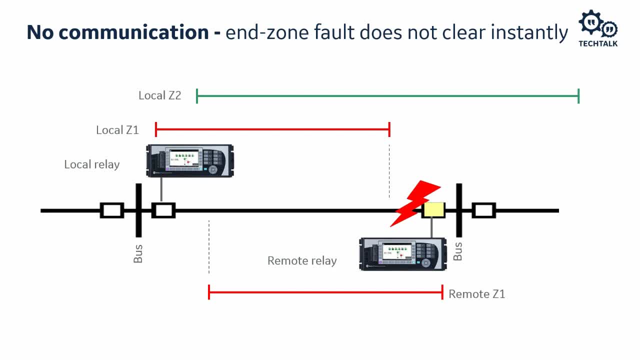 Line clearing must wait for the delay of Zone 2.. Of course the remote relay trips the remote circuit breaker instantly because this is in its Zone 1. The problem is that the fault still gets current from the local end until the local relay trips. 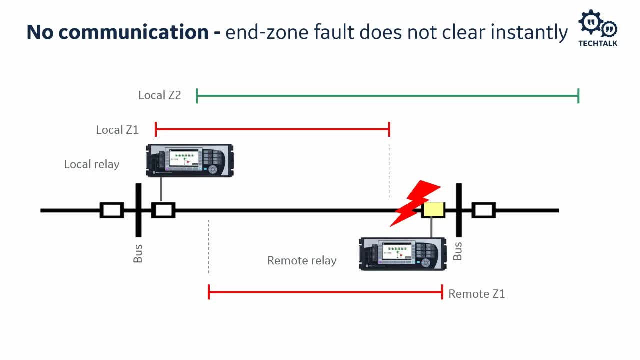 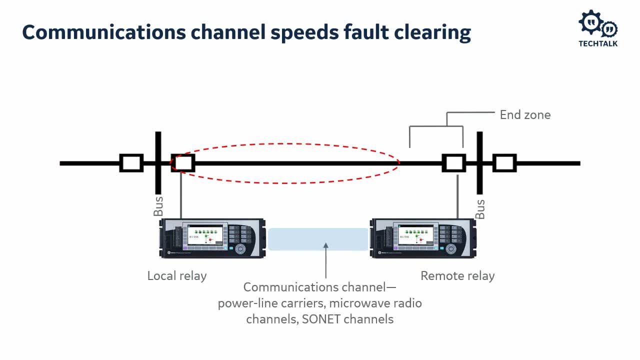 Without a pilot scheme we are stuck waiting until Zone 2 delay has expired. Then we can clear the line. A communications channel speeds fault clearing. Here is how it works. A fault occurs in the local relay end zone. The remote relay senses the fault and trips. 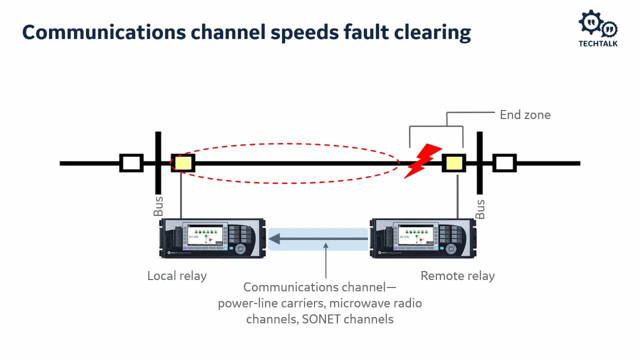 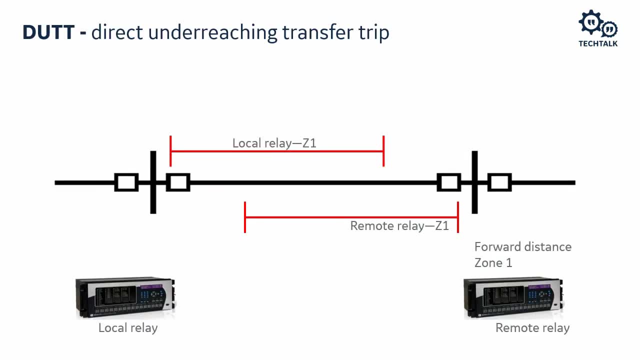 The remote relay sends the fault condition status to the local relay. The local relay trips, The line fault is cleared. This architecture is the simplest pilot aided protection scheme, DUTT Direct Under Reaching Transfer Trip When a fault occurs in the local relay end zone. 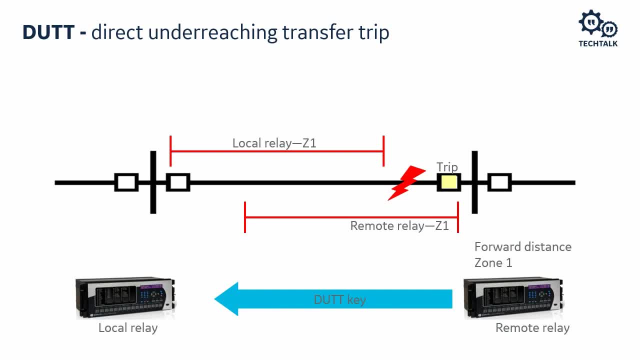 immediately, the remote relay identifies the fault in its Zone 1 and trips the circuit breaker on its side of the line. Also, the remote relay sends a signal, known as the DUTT key, over the communications channel to the local relay. This is where the term Under Reaching originated. 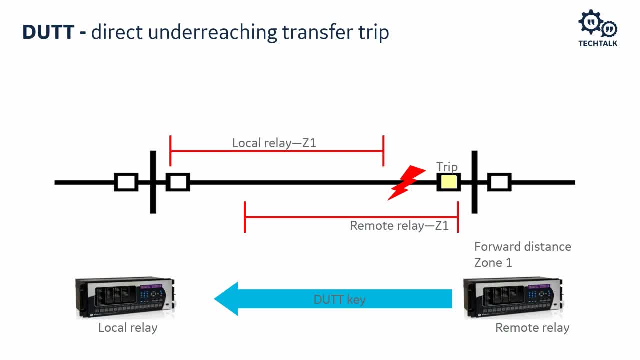 The keying signal is initiated by identifying a fault within the Under Reaching Zone: 1. As soon as the local relay receives the DUTT key, it trips its circuit breaker and clears the fault on the transmission line, The communications channel in a DUTT scheme. 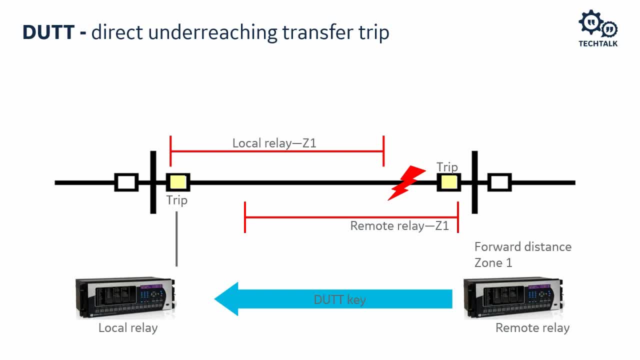 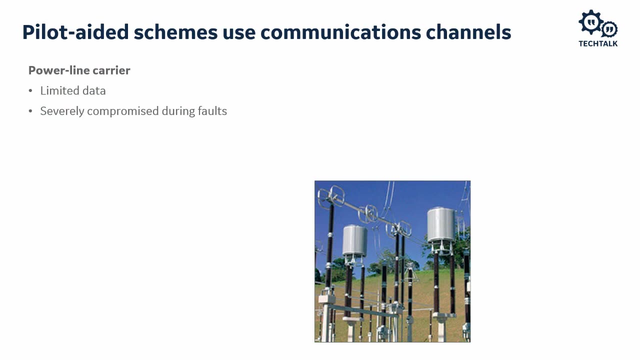 can have many configurations. All that is required is one bit of data. So a power line carrier communications channel would work as well as other types of channels. Pilot aided schemes use communications channels. We just spoke about a power line carrier, Special filters connected to the actual transmission line. 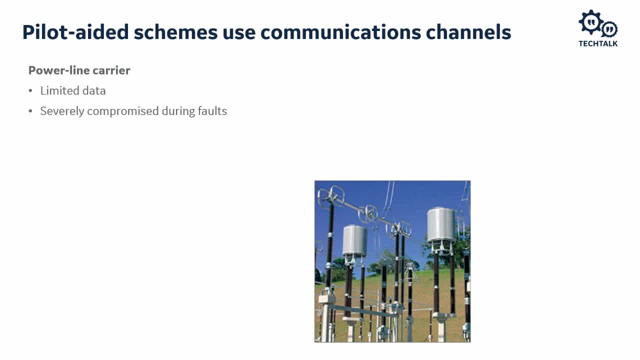 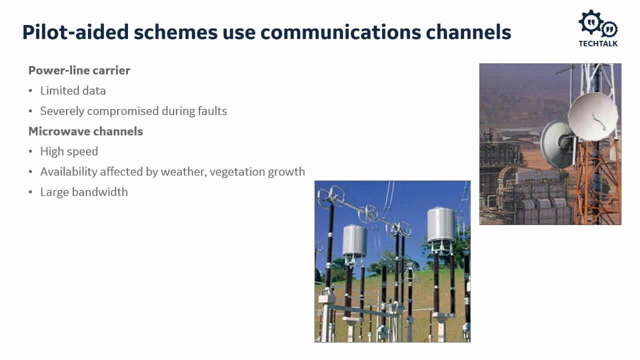 create a communications channel on the protected line. PLC send limited data and are severely compromised during faults. It is desirable to have a very secure and reliable communications channel for pilot aided schemes. Some modern improvements are microwave channels and fiber optic channels with attributes shown here. 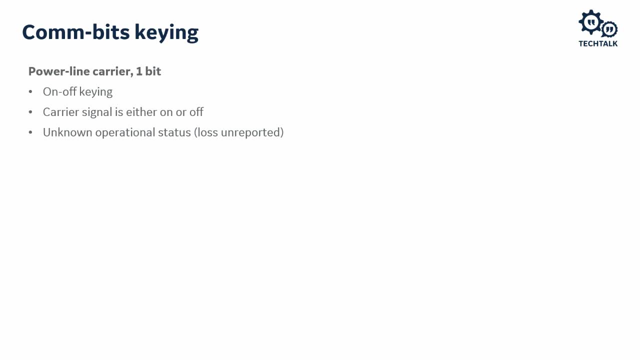 As stated, power line carrier sends limited data, only on-off keying and no status reporting. A channel can have two tones multiplexed on it, which is freaky, which is frequency shift keying. The two tones represent two bits: guard and key trip permission. 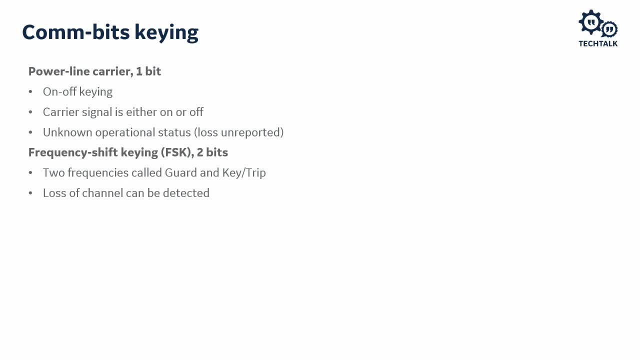 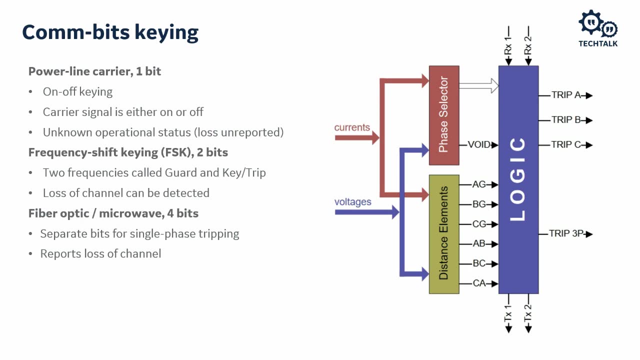 A channel loss report occurs upon the loss of the guard tone. Modern fiber optic and microwave systems can transmit as many as four bits. For example, single pole protection and tripping requires four bits of information and loss of channel reporting is included. We've discussed a simple DUTT scheme. 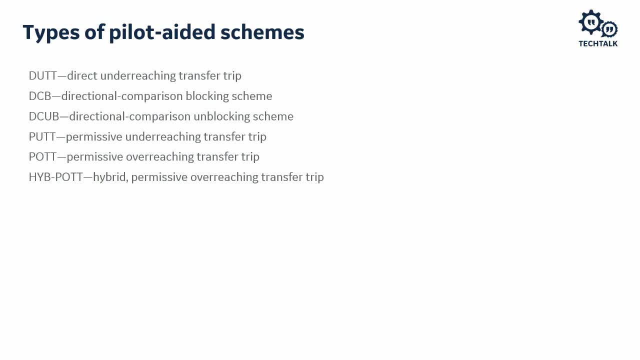 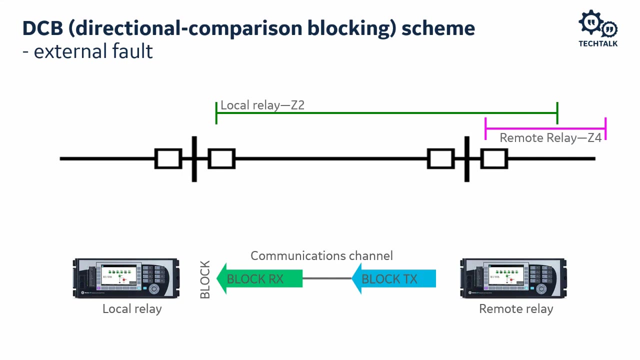 but here's a list of the other pilot aided distance schemes. These are combinations of blocking, unblocking and permissive schemes. Let's take a look at the directional comparison blocking scheme. In this scheme the local relay has an additional delay timer set considerably shorter than the normal. 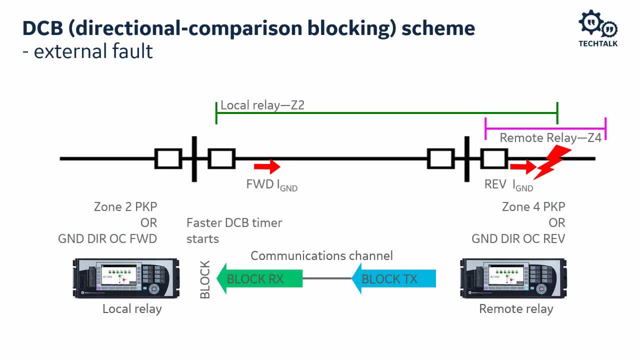 zone 2 delay. It is started by a fault detected inside its zone 2 area of protection or by ground current flowing in the third direction. The blocking signal remains intact. The remote relay detects an external reverse fault, zone 4, or ground directional overcurrent reverse. 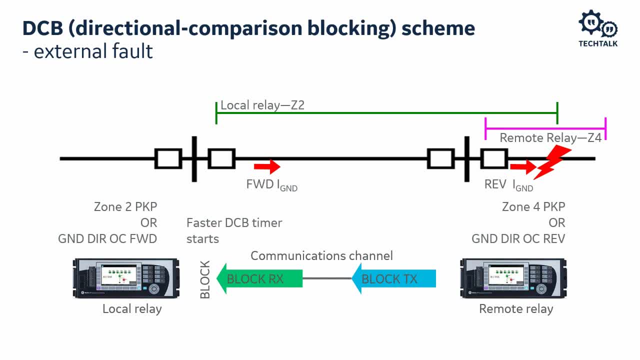 It does not trip and it continues to send the block signal to the local relay. The local relay DCB timer expires. It has the block signal and does not trip For an internal fault. the remote relay senses the fault trips the remote end circuit breaker. 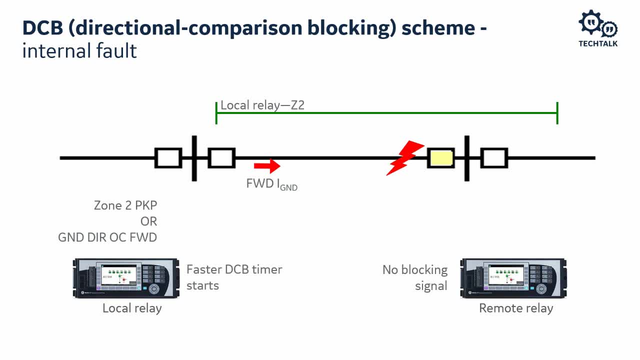 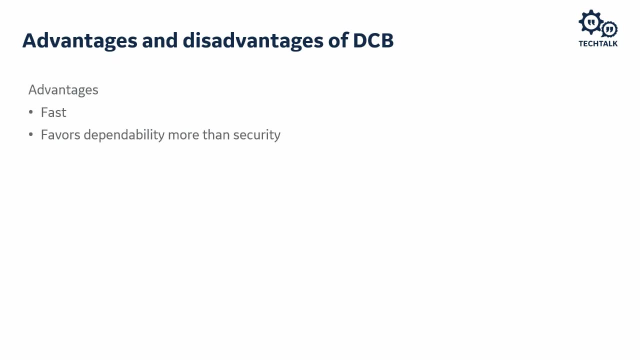 and stops sending the blocking signal When the local relay DCB timer expires. the local relay checks for a block signal. If there is no block, it trips the local circuit breaker. Advantages of the DCB scheme are that it's fast and it favors dependability. 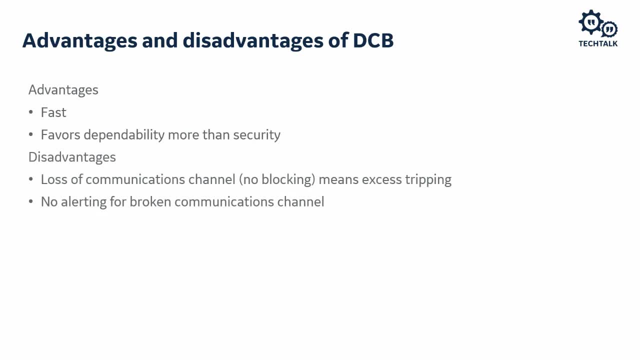 more than security. DCB disadvantages are: the loss of the communications channel means no blocking and that leads to excess tripping. no alerting for broken communications channel. Two channels are better than one, which is the next topic: DCUB. 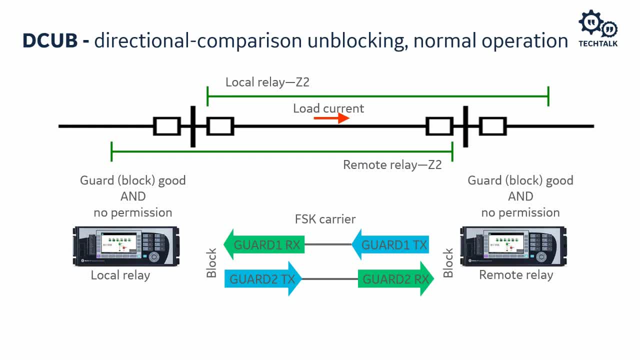 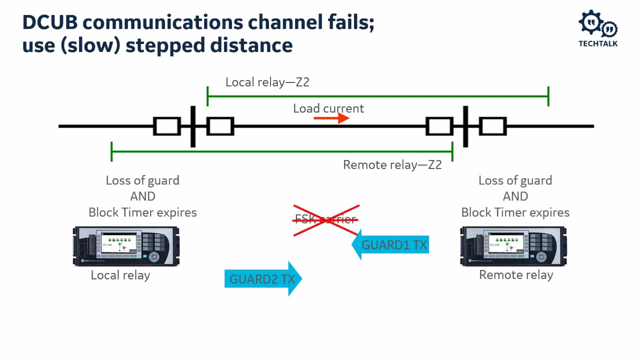 The directional comparison unblocking scheme operates reliably with two-tone FSK channels like power line carrier. In the directional unblocking scheme, the local and remote relays transmit and receive a guard or block signal continuously over the single FSK power line carrier In the event of the loss of the communications channel. 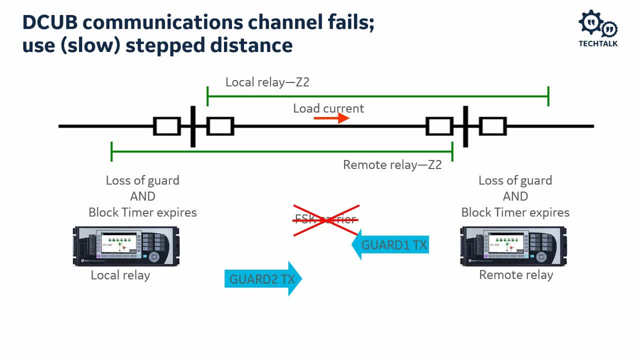 the local and remote relays try continuously to transmit a guard or block signal over the FSK power line carrier. However, the guard is not received, The DCUB block timer starts to time out and, when it expires, declares a loss of the guard signal. 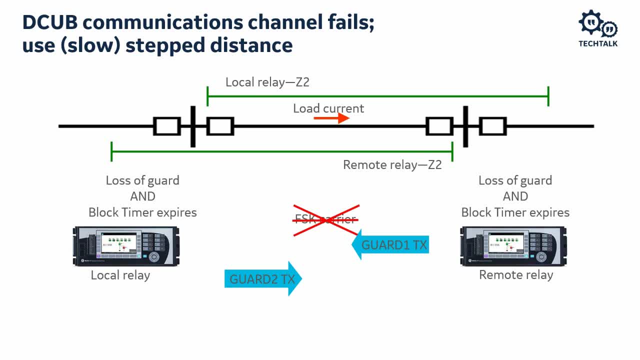 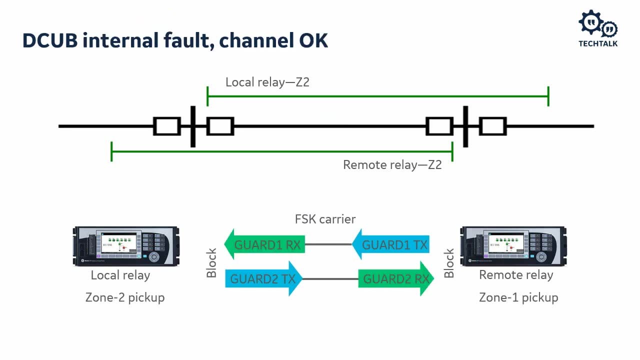 As a result, the DCUB scheme is disabled. With the loss of communication, the relays use the stepped distance protection scheme. DCUB operation returns when the guard is received by both relays. Here is the action when there is an internal fault. 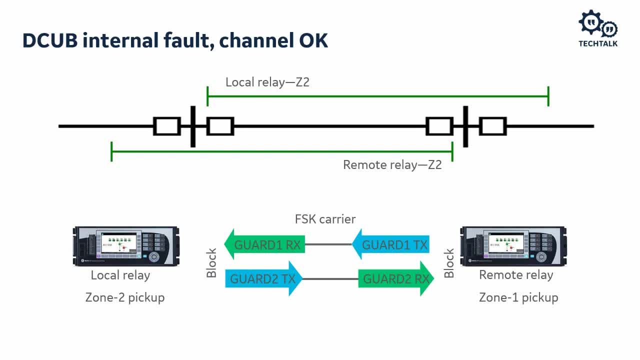 in the DCUB scheme and the channel is OK. The remote relay trips on zone 1 and sends the permissive signal to the local relay. The local relay notes the loss of guard signal and receives the permissive signal. It trips the local circuit breaker. 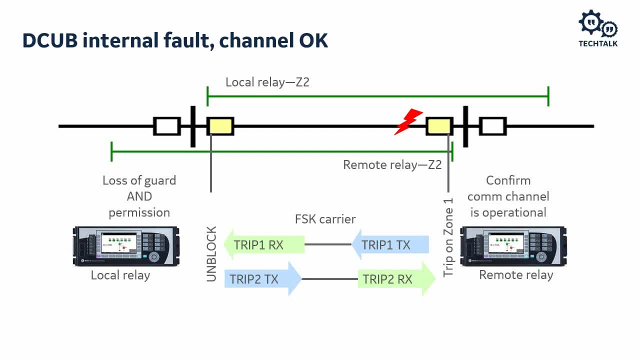 The local relay returns a permissive signal to the remote relay which confirms that the communications channel is operational. What happens with the DCUB scheme and a channel failure? In this example we see a loss of the communications channel. The DCUB block timer times out. 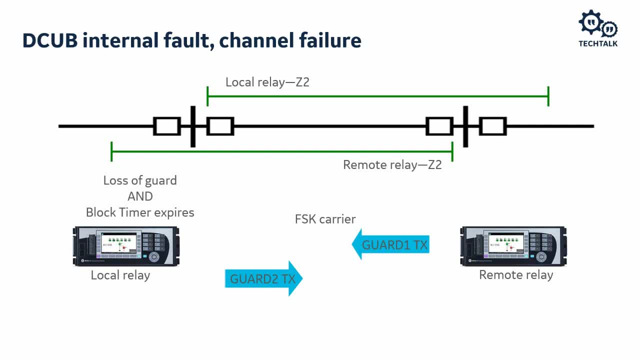 and declares a loss of the channel. When a fault occurs, the remote relay trips and sends the permission. However, the local relay does not receive the unblock. Without communication, the relay trips slower on stepped distance. The remote relay does not get a channel confirmation. 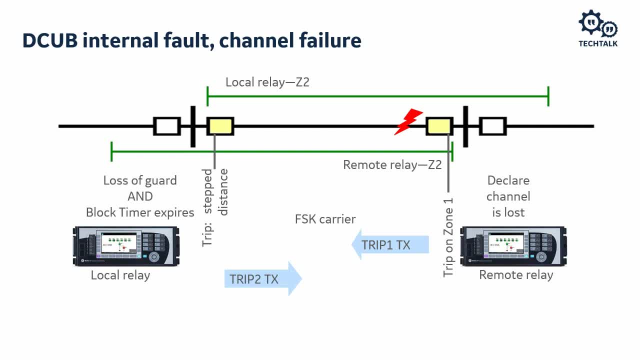 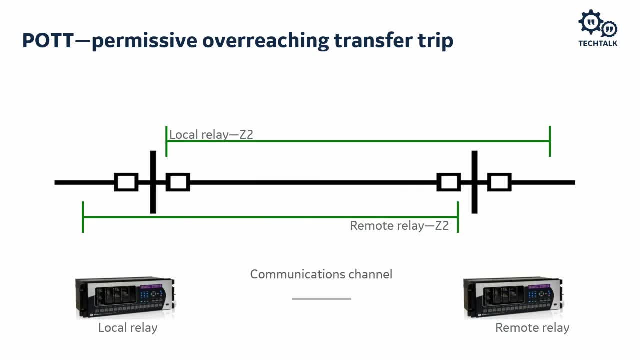 so it declares a channel lost alarm. DCUB operation returns when the guard is received by both relays. The POT Permissive Over-Reaching Transfer Trip Scheme is very popular. In the POT scheme we use two zone 2 elements and a communications channel. 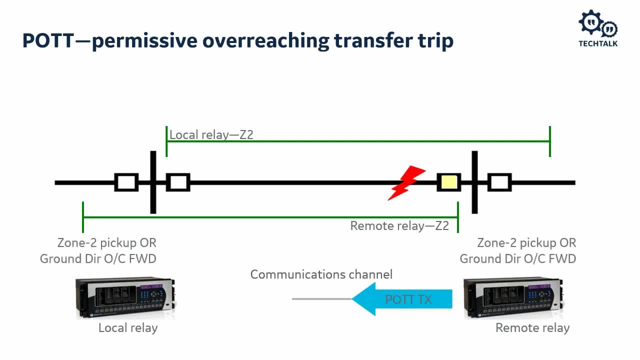 The local relay senses a line end fault with either the overreaching zone 2 or with a forward ground directional overcurrent. At the same time, the remote relay senses the fault and trips the remote circuit breaker. In addition, the remote relay sends the POTT key signal. 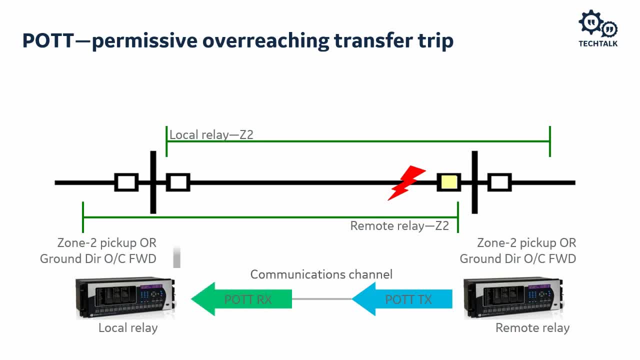 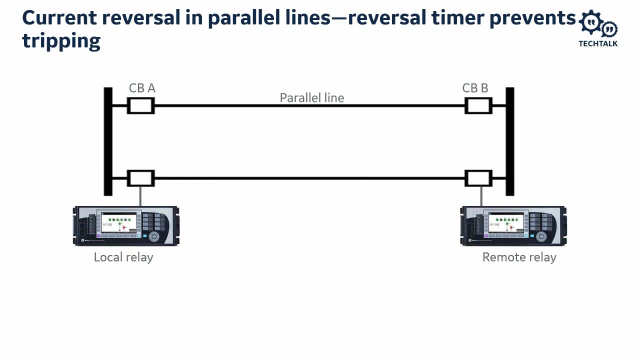 to the local relay. The local relay POTT logic receives the POTT key and trips the local circuit breaker. With parallel lines security can be a problem for overreaching distance protection. Additional logic is needed in the POTT scheme to provide extra security. 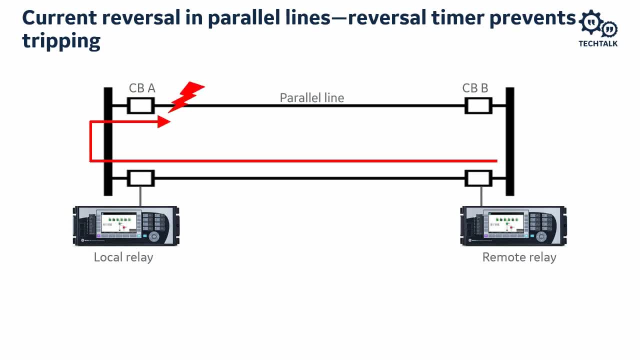 For example, if a fault occurs on the parallel, the upper transmission line, the remote relay detects forward ground current. It sends a permissive POTT key to the local relay. The local relay detects that ground current is flowing in the reverse direction. 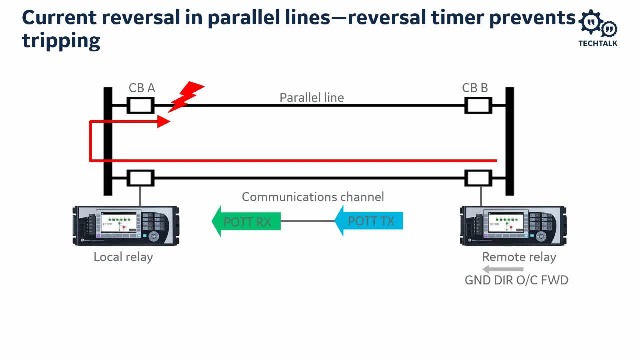 so it does not trip Circuit breaker CBA on the parallel line trips. and now we have a problem. Ground current begins to flow through the transmission line in the opposite direction. The remote relay senses a reverse fault and it inhibits tripping of circuit breakers. 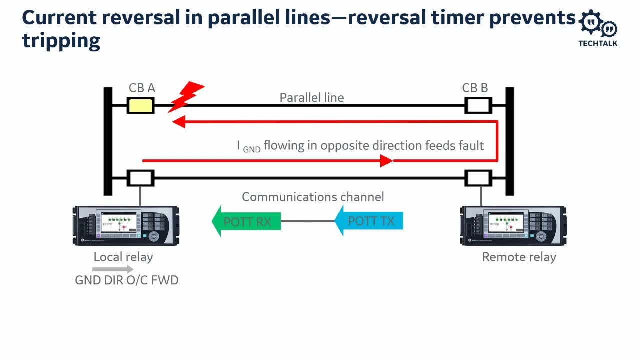 on the healthy line. However, the local relay identifies that the current is flowing in the forward direction and it might still have permission to trip if the reset time of the remote relay- forward-looking elements is longer than the operating time of the local relay forward-looking elements. 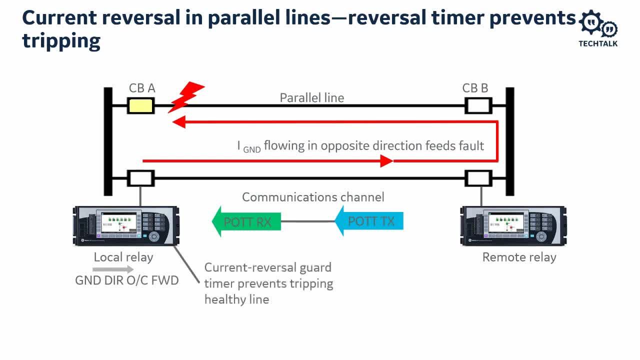 The solution Incorporate a blocking timer that prevents current reversal tripping at the local relay. This current reversal guard timer is initiated by the local relay's reverse-looking element that inhibits the local relay permissive trip logic. The delay in this timer must be longer. 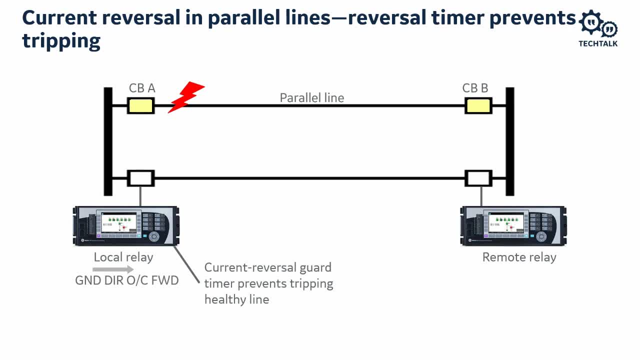 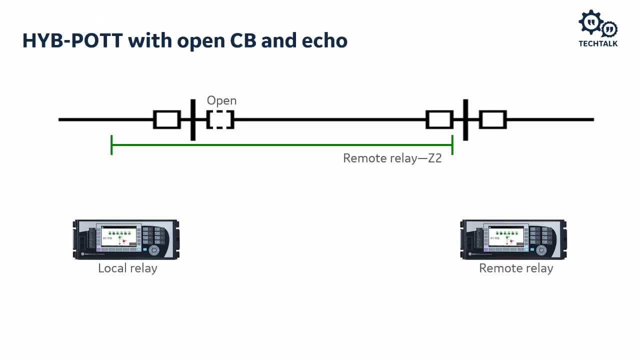 than the reset times of the remote relay elements. It gives circuit breaker CBB time to clear the parallel transmission line. A hybrid POTT scheme has both tripping and blocking attributes. Here we see a potential problem for the POTT scheme in that one end of the line is open. 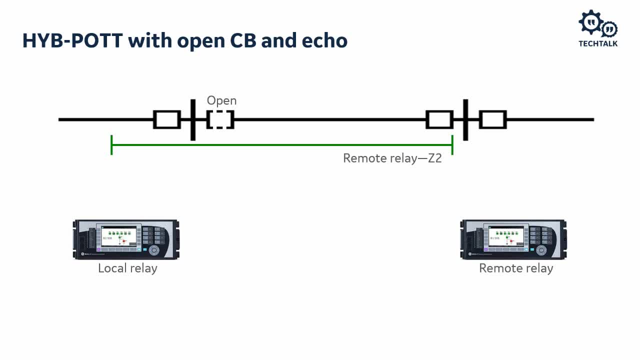 If the circuit breaker is open then the local relay does not measure current flow into the transmission line. It cannot sense faults within its zone of protection. If there is an end zone fault for the remote relay, it cannot trip until remote zone 2. 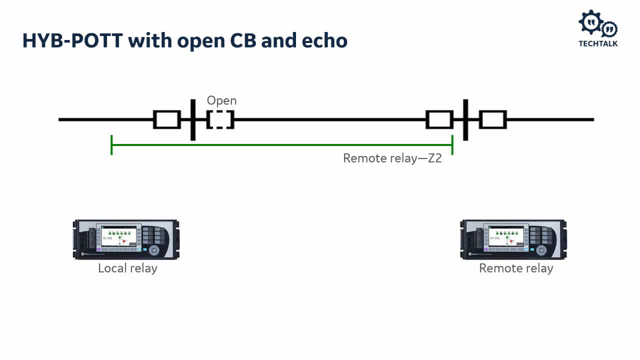 is timed out. There is no local relay POTT key. There is a way for the local end to send a permissive signal to the remote end. It's called ECHO. It speeds line clearing and then gets ECHO permission. It works like this. 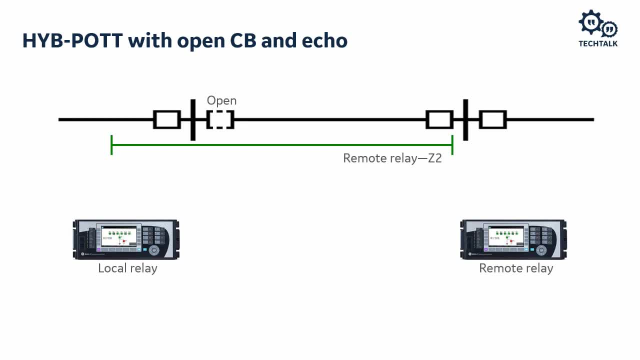 The local relay detects that its own circuit breaker is open and so it arms the ECHO logic. A fault occurs in the remote relay end zone. The local circuit breaker is open and the local relay receives a POTT key from the remote relay. Then the local relay sends or echoes back. 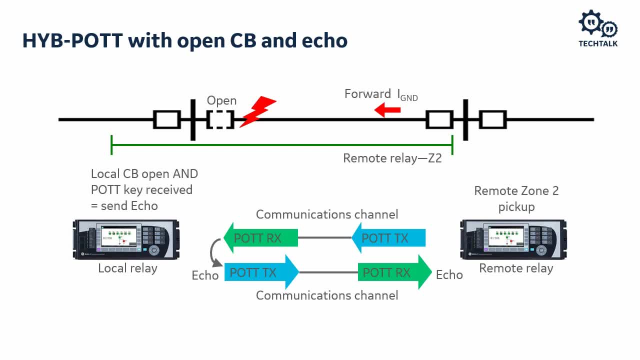 the received POTT key sequence directly to the remote relay. Next, the remote relay takes this echoed POTT key and trips the remote circuit breaker. This method clears the fault faster and ensures that the system does not become unstable. Tripping occurs in a weak-in-feed condition. 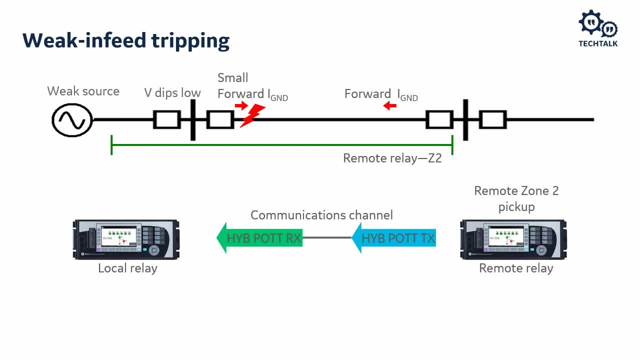 A fault occurs on the protected line near the local relay. Because a weak source feeds the fault, the voltage dips and the resulting current is small. The remote relay sends a hybrid POTT transmit signal. The local relay has no block. The fault is on the protected line. 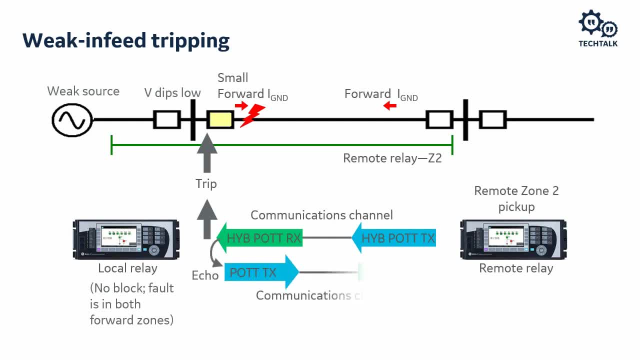 It trips the local circuit breaker. The local relay sends an echo signal back to the remote relay which trips and clears the line. Blocking also occurs in a weak-in-feed condition. A reverse fault occurs on the protected line near the local relay Because a weak source feeds the fault. 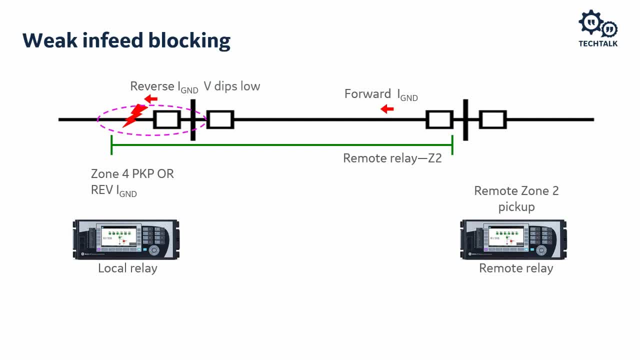 voltage dips and the resulting current is small. The remote relay sends a hybrid POTT transmit signal. The local relay has zone 4 picked up so it blocks. The fault is not on the protected line, That's it. No echo goes back to the remote relay. 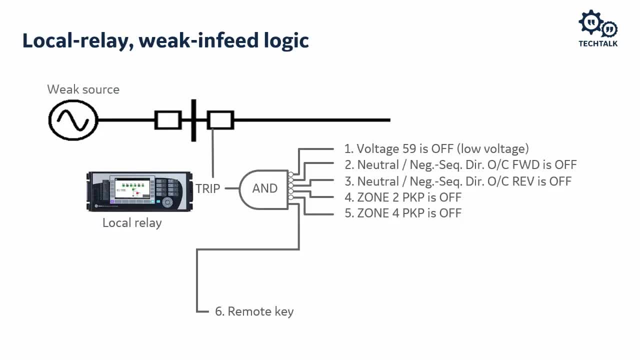 so it does not trip For a fault that's located close to the local relay on a transmission line with weak-in-feed. the weak-in-feed feature detects and clears this fault if all of the following conditions are true: Voltage has dropped close to zero. 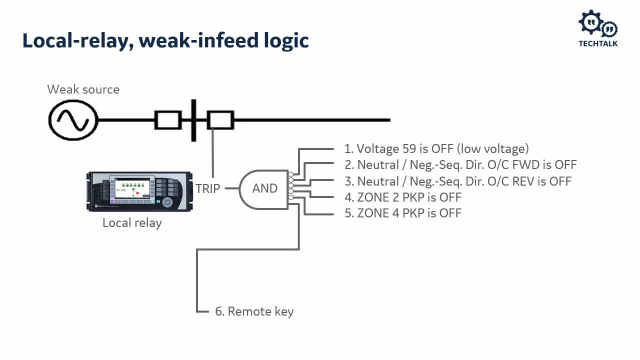 Forward and reverse directional overcurrent protection elements have not picked up. No faults are detected in forward zone 2 and reverse zone 4.. If all of the above conditions are met and if permission is received from the remote relay, hybrid POTT key, 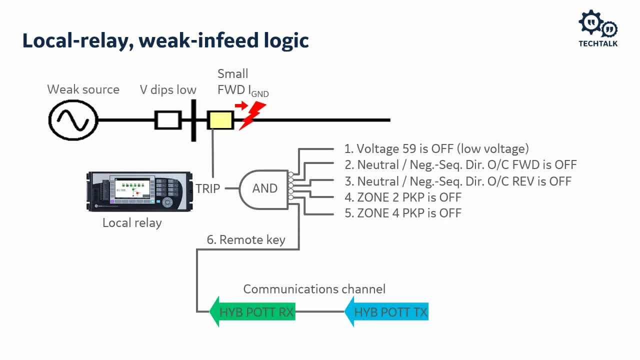 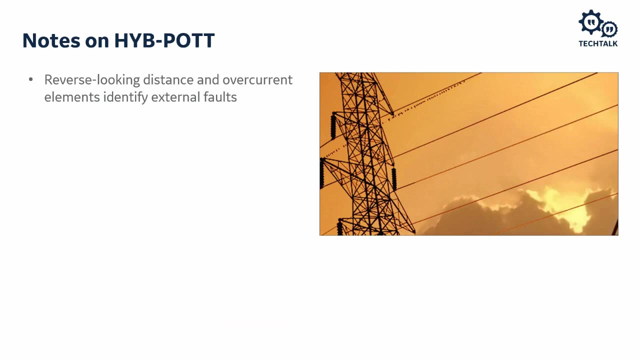 then the local relay hybrid POTT scheme identifies these conditions as a fault that is being supplied by a weak source. It forces the local relay to trip the circuit breaker. Here are some things to remember with hybrid POTT schemes: Reverse-looking distance and overcurrent elements. 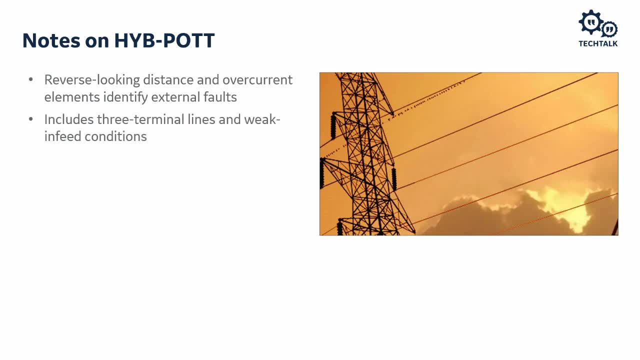 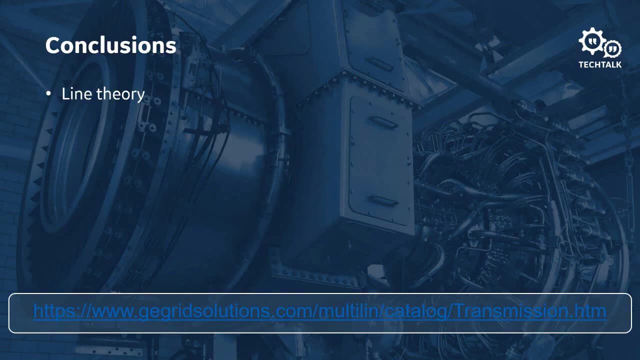 identify external faults. It includes three terminal lines in weak-in-feed conditions And the echo feature adds security during weak-in-feed conditions. Now it's time to conclude this presentation. In this session, I presented line theory, classifying lines and exploring impedances. 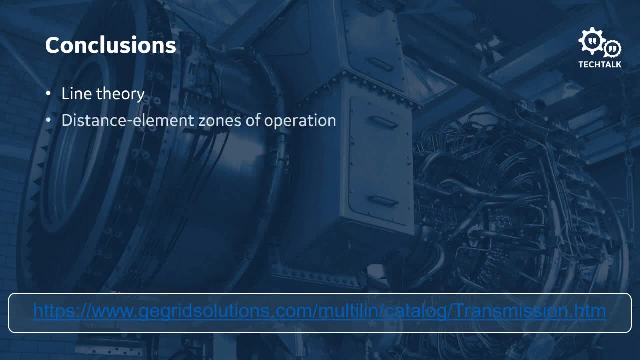 Next was distance element, zones of operation, Impedance, admittance or MO circle, reactance resistance and quadrilateral operation zones. I covered the MO zone in detail, including settings, resistance coverage, polarization and memory expansion. Applications discussed were pilot-aided. 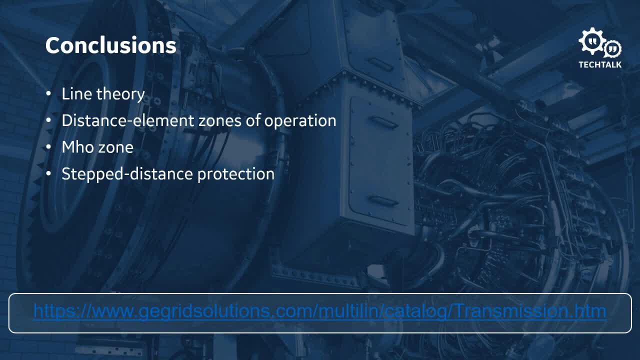 and non-pilot-aided schemes, and stepped distance protection with three forward zones and one reverse zone. Finally, I demonstrated pilot-aided distance schemes: DUTT, DCB, DCUB, POTT and hybrid POTT. Now it's time for your questions. 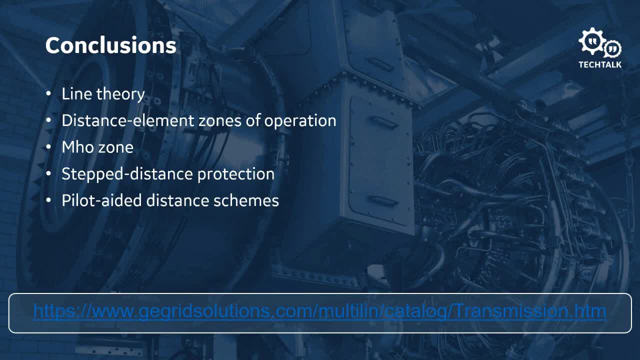 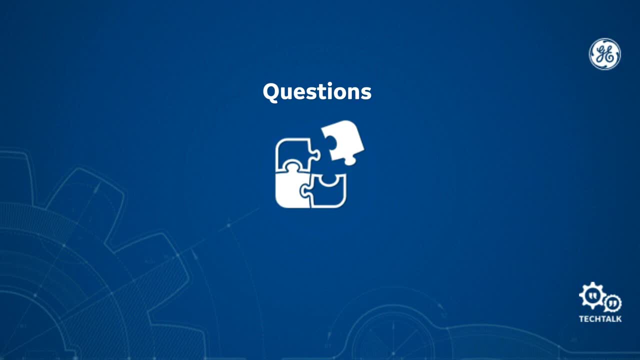 Just a reminder that if you'd like to submit a question, please click the Q&A widget at the bottom of your screen, Type your question in the text field and click Submit. Dan, I'll turn it back over to you to begin answering the questions. 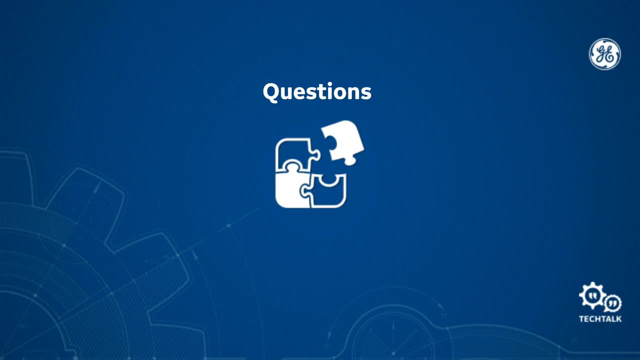 that have already come in. Now we're in the questions-and-answer, the Q&A period. taking a look at the incoming questions, Here's a good one: What is the difference between power swing and out-of-step protection functions, and how do you set settings for power swing? 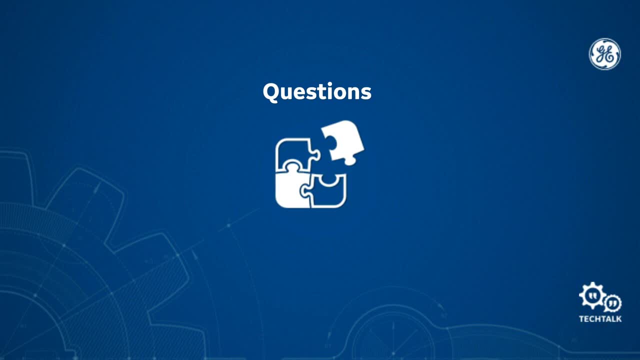 Well, at GE we call it power swing blocking and out-of-step tripping, and these can help stabilize a power system swing. A stable power swing is a condition where the system loses synchronism with the neighboring system for a short period and then later regains synchronism. There's two reasons that can cause this type of stable power swing. One of the systems loses a significant amount of generation and instantly becomes much weaker, but the system load remains constant or load suddenly increases substantially on a weak system, So tripping would occur. 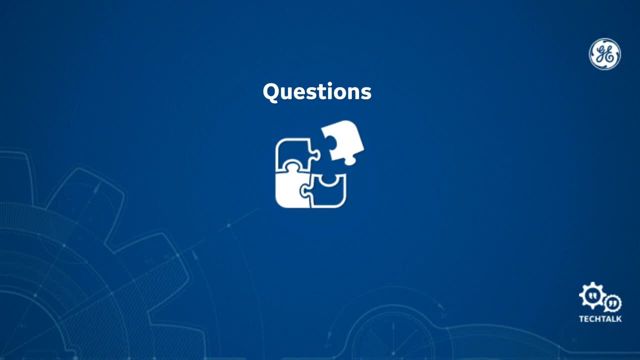 when the relay detects an unstable system. Too much time has passed while an impedance locus is in the protected zone or area, So that we would call out-of-step tripping. Different protection elements respond differently to power swings. If tripping is required for faults, 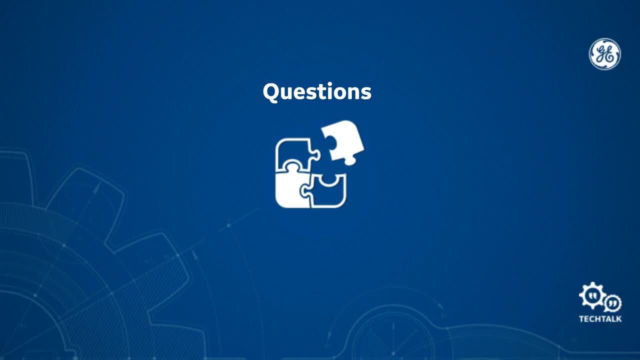 during a power swing some elements can be blocked permanently using the operand power swing block. Other elements can be blocked and dynamically unblocked upon fault detection. That would be the power swing unslant bar block operand. So during a power swing the voltages and the currents fluctuate. 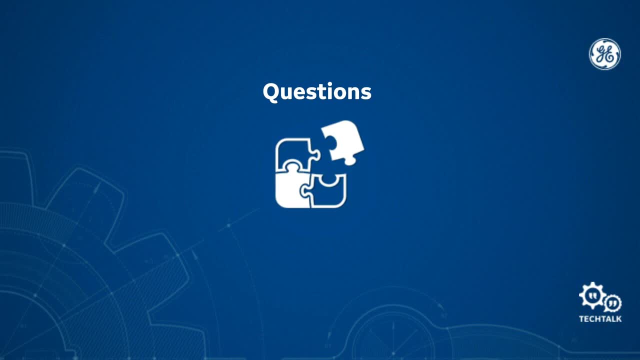 which significantly affects the value of the measured impedance of the line. Remember that our impedance locus is basically Z, or Zed equals V over I. So just before the power swing starts, we've got a large voltage and a small current. That would be normal load. 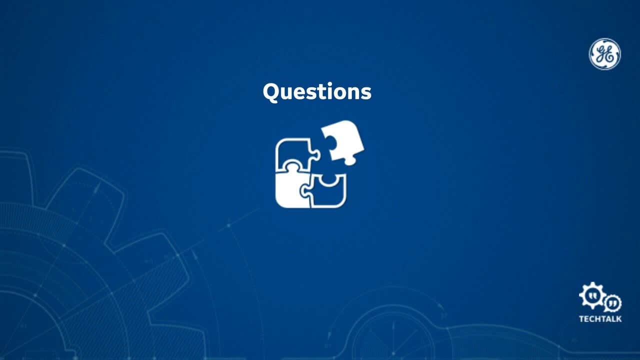 And then the swing starts. so either we lose the generation, as I said, or we get a bigger load. the plotted impedance moves slowly from the load point into the distance operating zones. It goes through the zone and then back out to the load point. 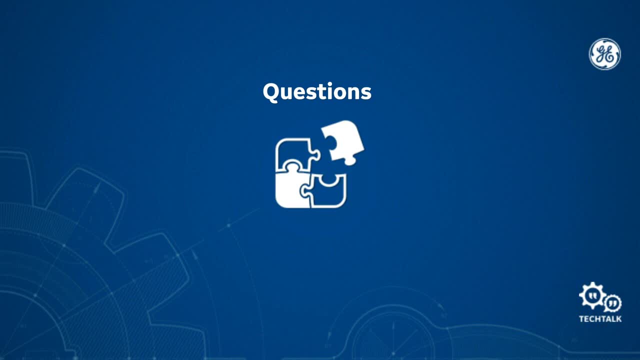 where the system regains synchronism. This would be a stable power swing. so we'd have blocking And the power swing blocking feature detects that the swing is recoverable and the distance zones don't operate. If you've had a bad day, 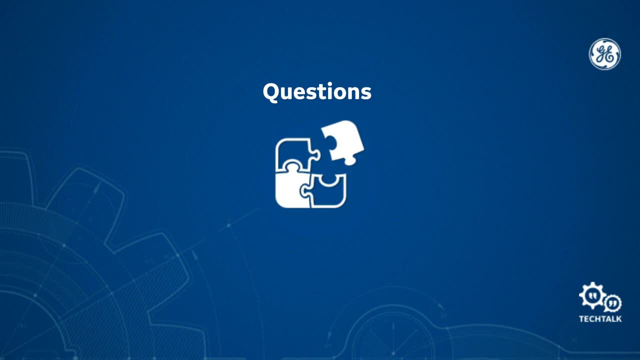 then things can get a little bit different. But we'll talk about tripping in just a moment. So a little further dive into blocking. we can set MO zones, Impedance zones or quadrilateral zones, either one, And we can define them. 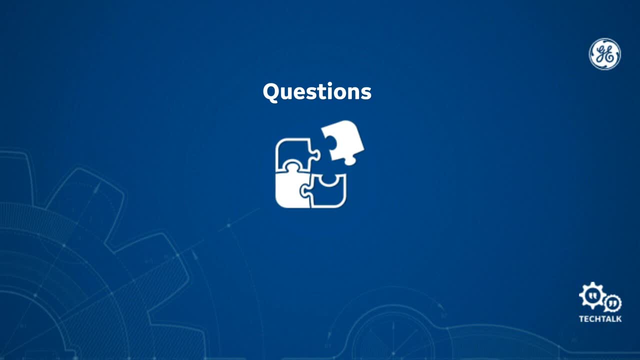 inner and outer blinders and middle blinders, depending if you use two or three. So the outer boundaries of the large. If you saw the tomato drawing, that would be a thing you could think about. So then you've got your inner, middle and outers. 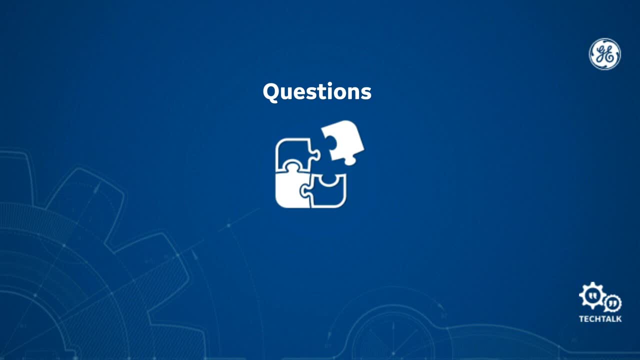 A timer starts when the impedance locus moves in to the outer one. We keep timing as it goes into the inners, which you can think of as maybe, if you're imagining two tomatoed MOs as the lens part, And then if the swing keeps swinging, 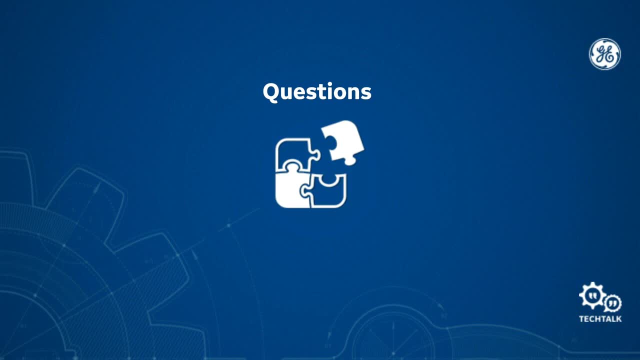 and goes out and crosses back in or crosses back out into the zone where we cross the outer, then we would have stable. The bad day starts when, if it's a real fault and you're not going to be able to recover the timers time out. 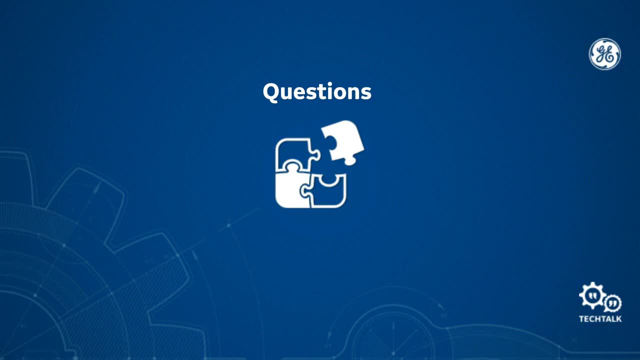 The locus stays inside the protected zone, And so then, instead of power swing blocking, we'd have out-of-step tripping. Let's see, here's a good question: What's the maximum latency that can be expected from teleprotection equipment for this scheme to operate properly? 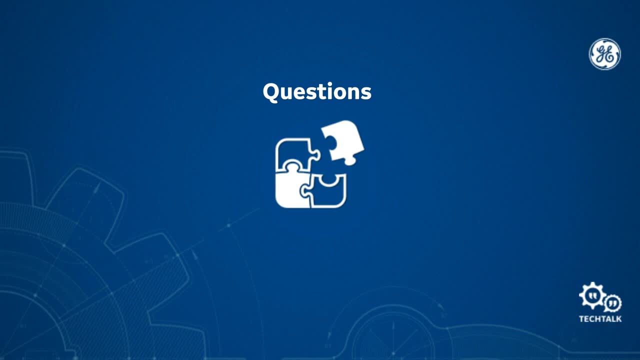 Well, it's like it is in the power and communications world: It depends. Power line carrier is still very, very popular, And the newer forms, the microwave and the fiber optic, are coming up. Each of them has their advantages and disadvantages. 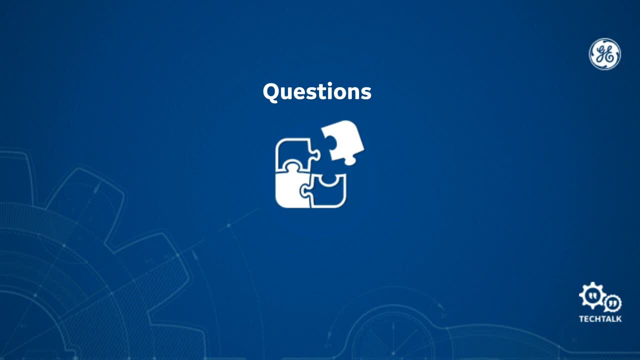 I would say you're looking to have about a five millisecond latency in the line. Now that adds to the latencies of if you're using physical relay closure contacts. as they slap together you've got maybe eight to 10 milliseconds, So that end-to-end channel time. 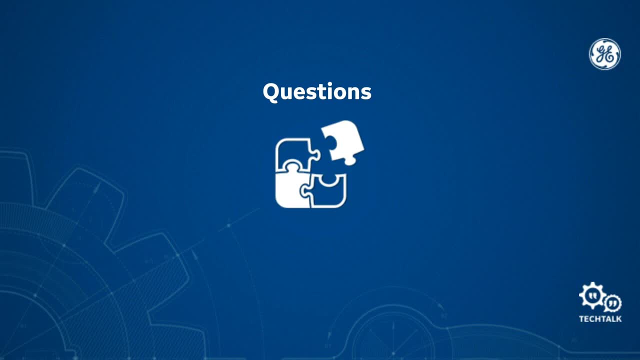 is going to add to that. Also, your circuit breaker times. you know really fast breakers. three cycle breakers or more is your overall clearing time for the fault. If you can stay under a cycle, you're really, really, really good. 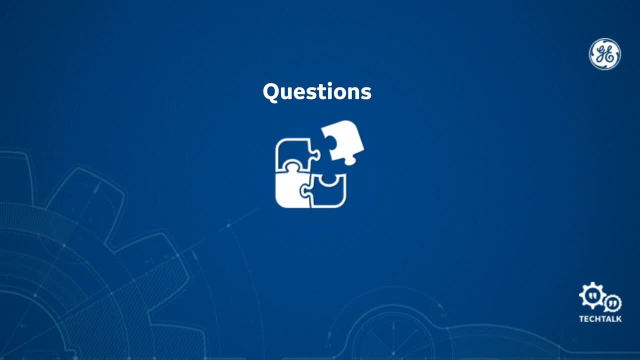 But mostly we're going to see five to 10 cycle clearings In regards to how fast the relay can detect what's the latency in the relay. So I've moved away from the channel to the relay. The multi-lin UR line is about a cycle and a half. 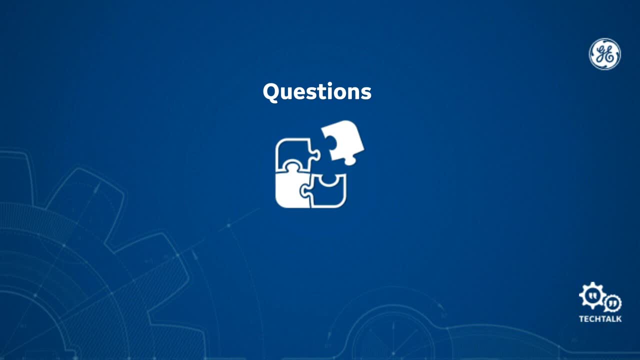 The micoms, which are wonderful technology. we're putting that technology into the UR lines. Those agile relays are sub-cycle tripping And that will be in the UR8 series when that comes out soon. Fast is good Because our task, as I described earlier. 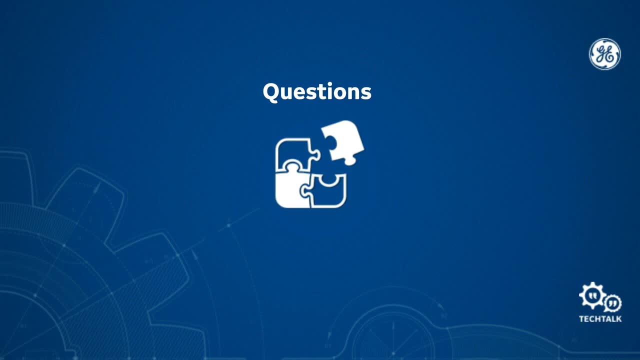 our job is to clear faults quickly. So here's a question. This is a good question, And we see this a lot now with our new grid, the way it's configured, Will distance protection work with inverter-based generation such as wind farm? 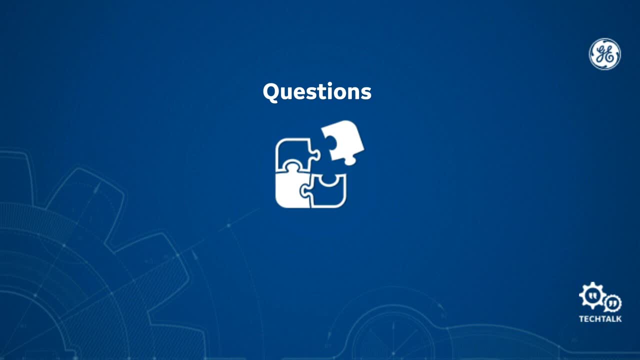 So I live in eastern Washington and it's beautiful. I think it's incredibly fantastic to drive around in a wind farm And see all the big wind farms, especially when it's just converting over to dusk And all of the little red lights are blinking. 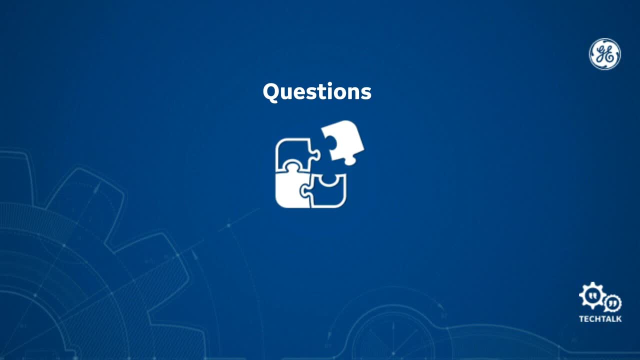 all at the same time on the horizon. It's a beautiful sight. All right, So we'll get from the aesthetic now into the actual physics. So wind turbine generators, WTGs. there are different kinds of them, And the fault output of these varies as per the type. 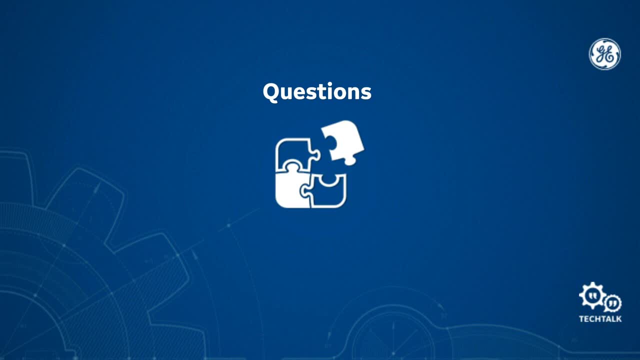 Most inverters, most wind inverters, limit current to a small value, about one to two times the full output, for a fault which can be a challenge for your distance elements And some of them, the type four inverters, produce balanced unity power factor currents. 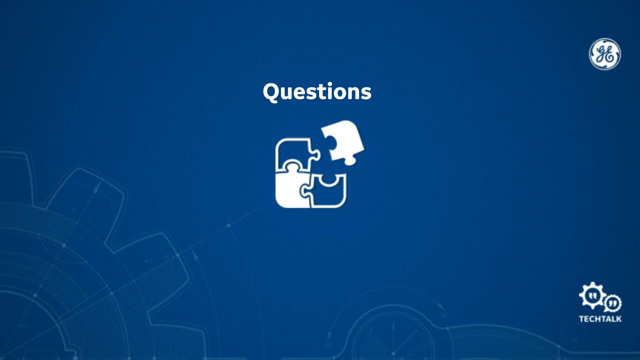 in response to an unbalanced fault. So I'd say that you've got a big challenge there with inverters and there are some great papers and we can do a whole other webinar on just how to protect with inverters, But there are signals that you can take out. 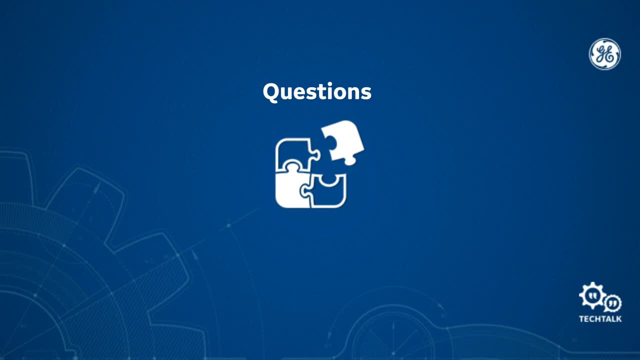 as transfer trip signals or communication signals from the inverters. that'll help you in getting a distance protection that works. It's a big topic. Here's another question. I didn't cover it and so thank you for asking the question PUT. 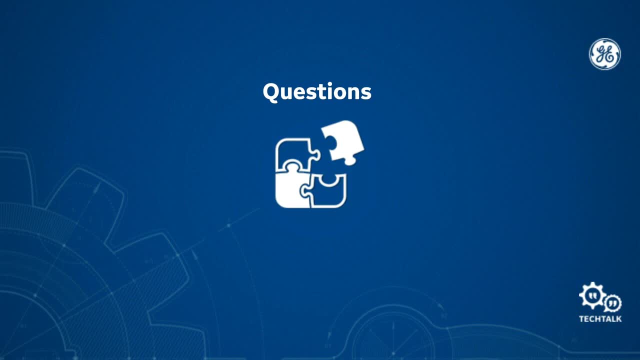 So I think I showed it on the screen, but I didn't talk about it. Permissive underreaching transfer trip. So what's the difference between PUT and POT? Permissive overreaching transfer trip. So permissive underreaching transfer trip. 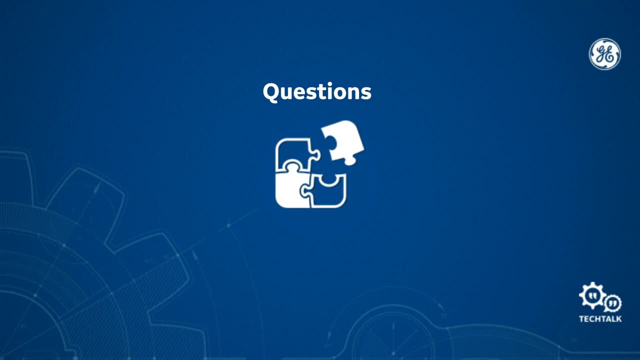 is a scheme where, just like POT, a key is sent between the two ends. But what differs? the thing that's different between the two schemes, is how you sense the fault. So in the underreaching scheme, the local and the remote relays. 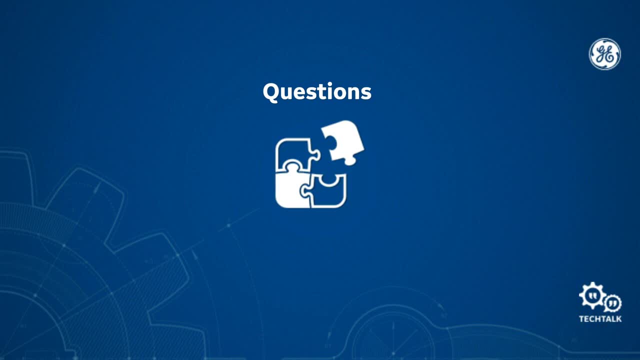 send the key only for local faults within the zone 180% reach With POT. of course both ends are overreaching, so you've got a little bit more coverage. The advantage for PUTT is that current remote relays, the current reversal, is not a problem. 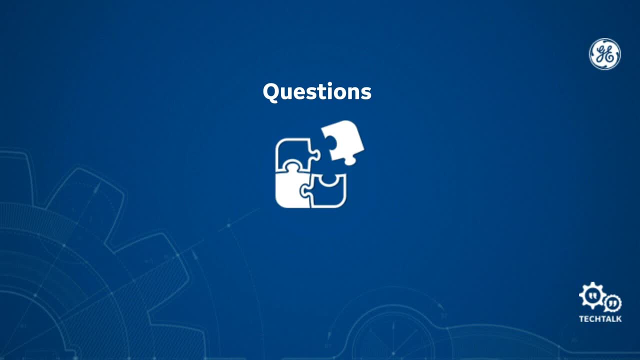 because, again, you're not using an overreaching element. So because zone one does not overreach, it doesn't have that problem with the current reversal that I talked about in the POTT scheme. So always good to have current reversal working in your POT scheme. 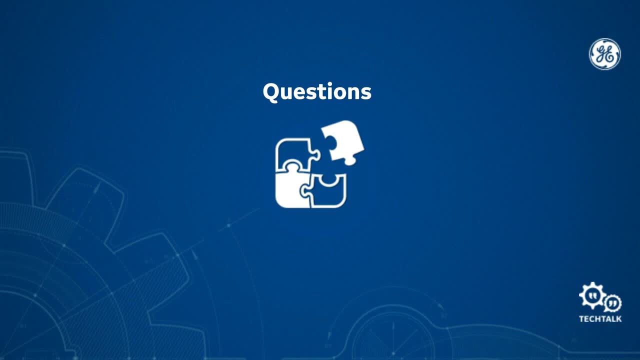 not really necessary in the PUTT scheme. You know PUTT isn't used very much because you need to have that overreaching detection on both line ends in the scheme. That's really why it's so popular. Here's another good question. 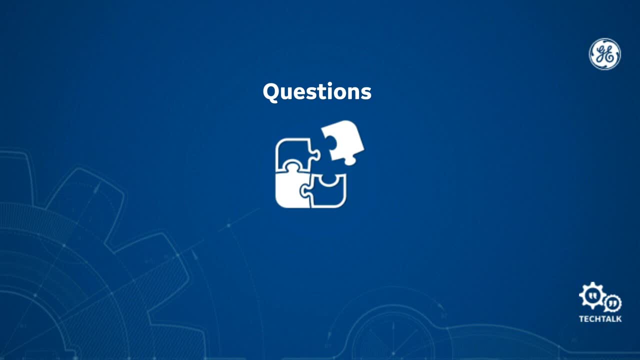 How do I protect short lines where the line distance protection zone covers a transformer? So often on short lines you'll want to include the transformer in the distance protection And in the old days we used to say no, no, no, we can't do that. 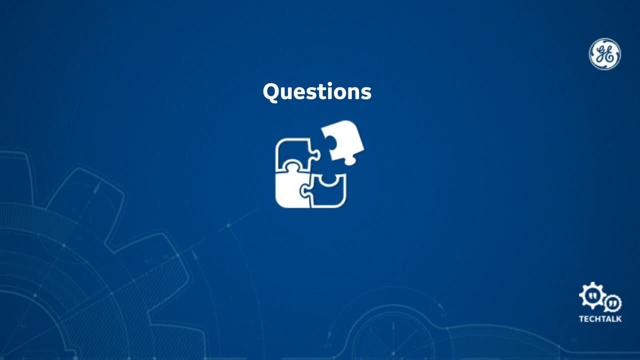 And now in the new days, in the modern era, we have the calculation power in the relays to actually do a little bit of compensation, connection, compensation y delta in the phase and also the ratio compensations. So because the relays compute the reach, 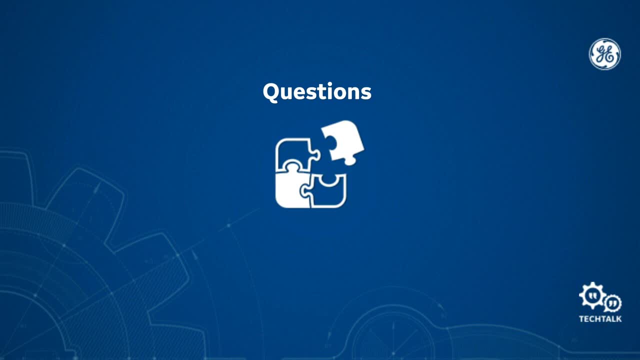 and take in the transformer impedances and the compensations. you're going to have to follow some rules when doing a transformer in a distance zone on a short line, So you got to think about secondary ohms. convert the transformer in the VTs. 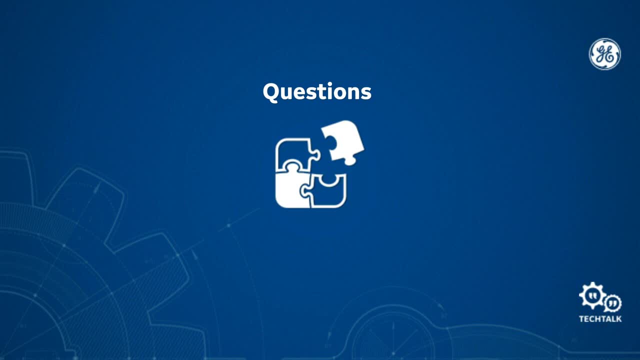 and the CTs as well and enter that into your calculation. You have to think about, in the zone you're covering, where are the VTs and the CTs? So the question is: in sensing the fault, do you have to look back? 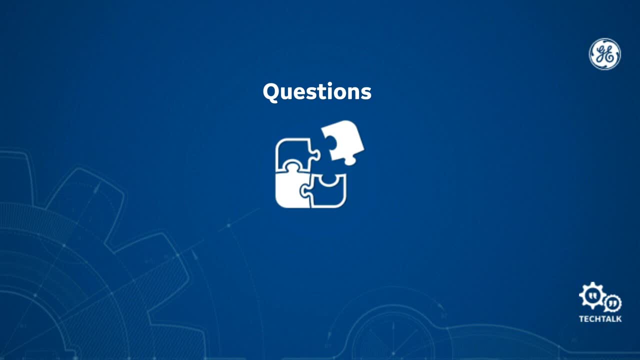 through the transformer to get the data from the VT. Do you have to look back through the transformer to get the data from the CT, And if so, then you'll have to include those in your calculation. There's a number of ways to do this. 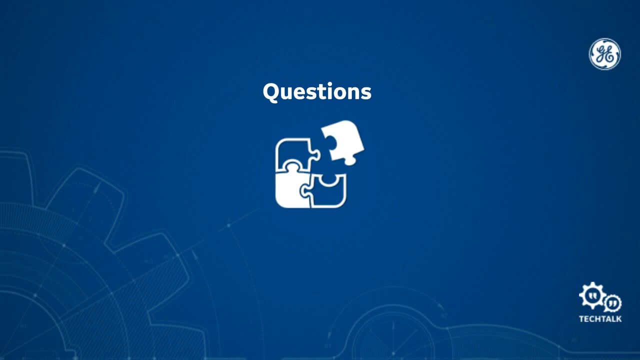 And the UR manual has a great treatise on this And if you email me, we can talk about this some more. But the idea here is that again you think about the fault and how the fault is being sensed, what PTs and what CTs sense it. 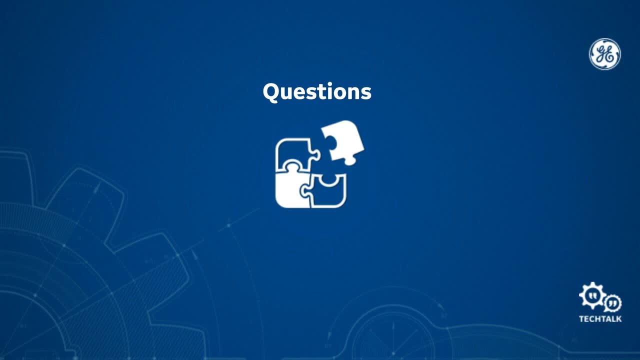 and whether you need to apply the transformer compensation to that ET or PT signal so you can accurately represent the transformer in and out of the zone. Usually you've got a forward zone with the transformer and a reverse zone without the transformer. There's some great applications for that. 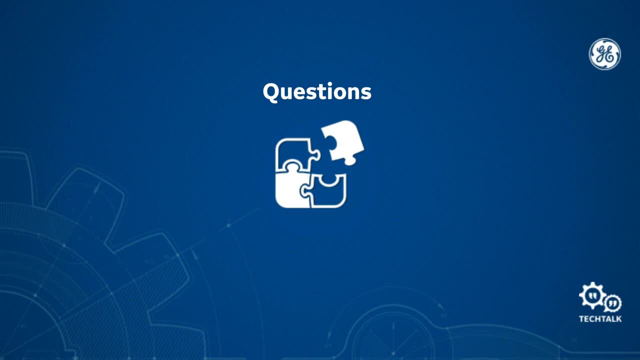 Take a look at another question here: What's? Oh, this is interesting. I didn't talk. I talked a little bit about power line carrier in the presentation. What's an easy method to calculate modal analysis in a transmission line for power line carrier? 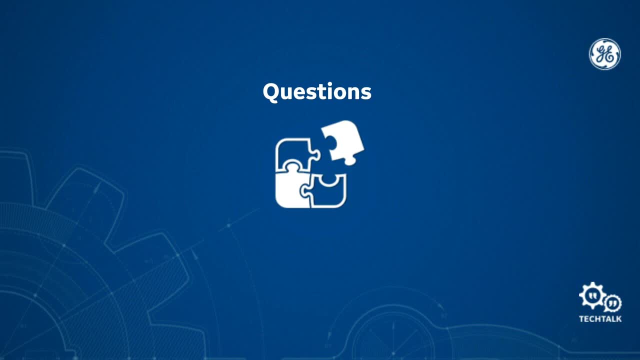 Well, that's kind of the wizard big tall hat. Modal theory in power line carrier states that there are independent propagation modes on a transmission line. Think of a three-phase line across country. So if there are three ABC phases in the line, there are three modes. 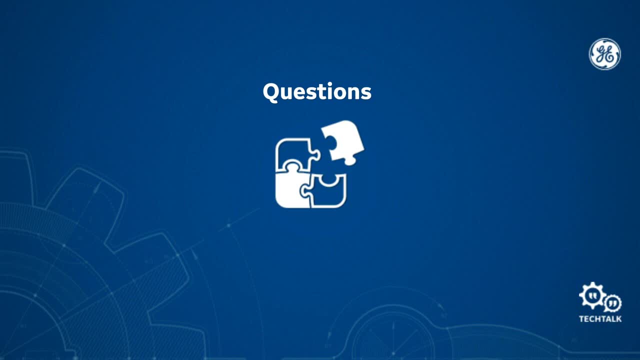 or modes, kind of like symmetrical components, where you've got I1, I2, I0.. In modal theory, for power line carrier, you've got mode 1,, mode 2, mode 3.. Mode 1, is where we go out. 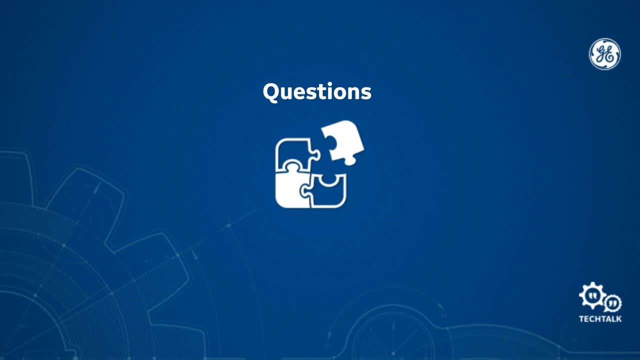 or send out on the outer phases and we come back on the middle phase. Notice I didn't say we go out on A and C and back on B, because on long transmission lines we transpose. I'll talk a little bit more about transpose in a second. 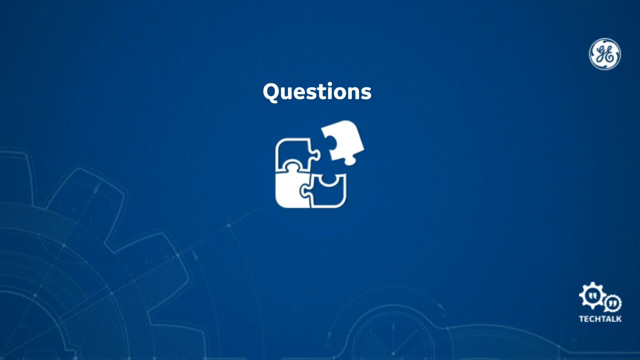 On mode 2, you go out on the outer phase and come back on the other outer phase And mode 3, you go out on all the phases and you come back through ground. And everybody knows that ground is lossy, so it's not very effective. 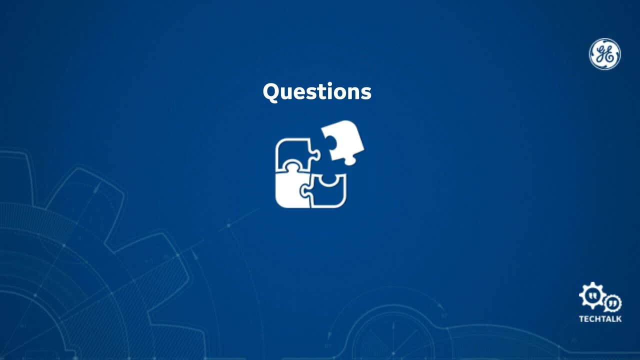 compared to the other two. I mean you can use it but you're limited to about 10 miles And that problem of line transposition really complicates the modal analysis. I've done this by hand. It takes days because every time you transpose 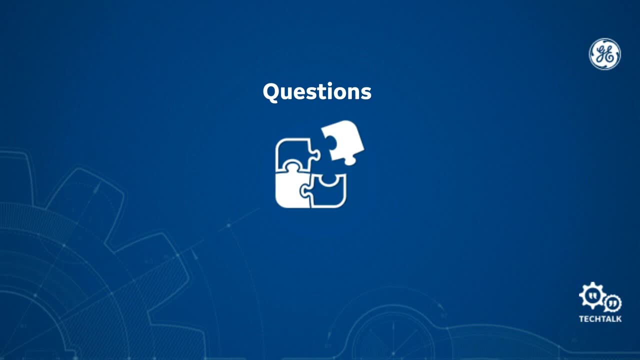 you've got to do all your calculations all over again, And so really the best way to go is that these days we have an app for that. There's some really good software that makes the modal analysis a lot easier and a lot faster. 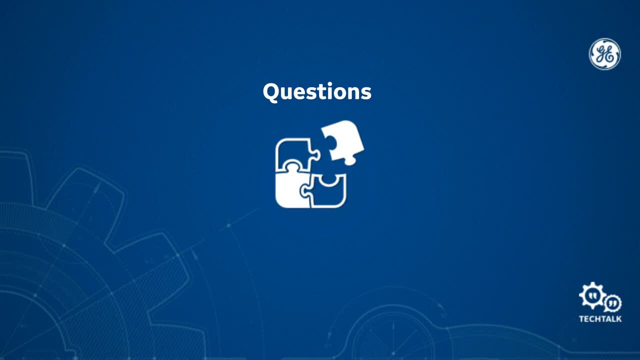 I'm a big fan of hand calculation and I still use my HP48G every day. reverse Polish forever to enter. 2 plus equals 4.. Got to love that. Let's see. Here was a question on why do we use resistive zone. 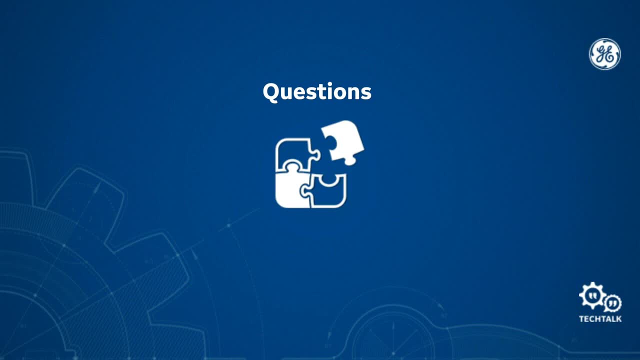 to get reactants. and why do we use a reactant zone to get resistance? It's kind of a weird English thing, right, Because they all start with re. So the resistive zone being that it's kind of up and down or vertical. 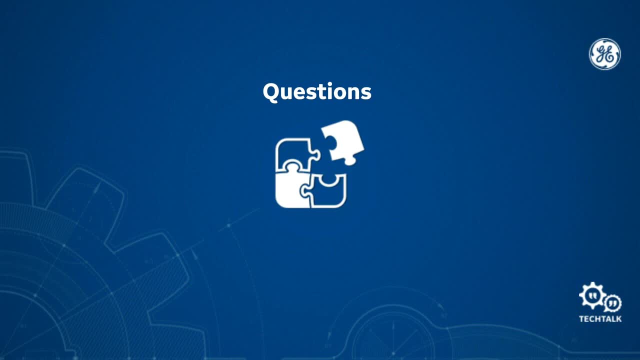 We can pull in those blinders and it's very similar to blinders you'd use on out of step, And so that would determine how much react if there is reactants close to the line, And the reactants coverage then tells me how much out. 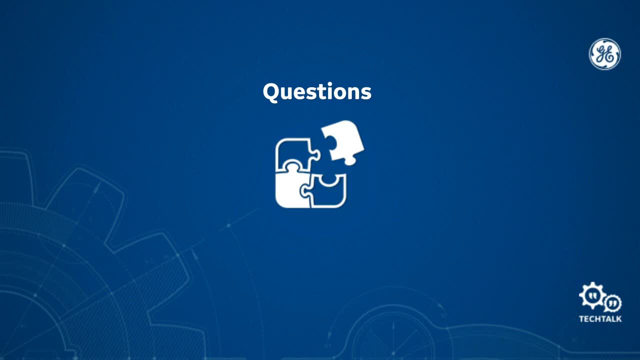 how much horizontal. if you're thinking of the RX diagram. Yeah, it takes a little bit to wrap your mind around that And I think that if you take a look at those slides as we send those to you and think about it, I think that will help you. 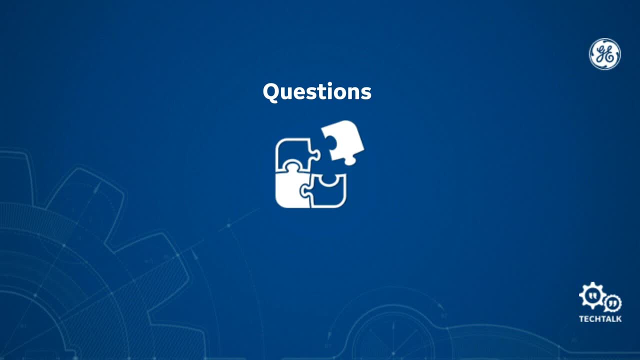 Let's see We've got another question here on series compensated lines. That's a big topic. Series compensated lines would be the whole webinar we could do on series compensated lines, But just to give you the quick basics of that. So on a very long line, 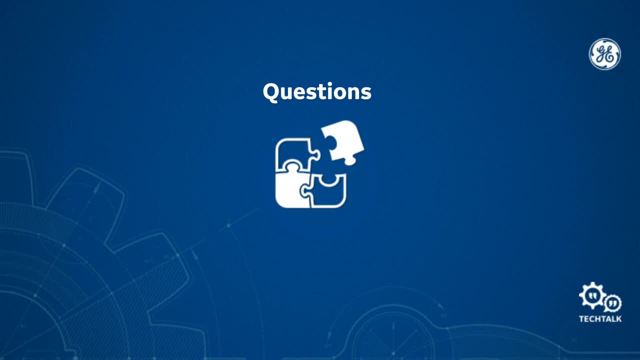 you've got a lot of reactants, inductive reactants. that makes it pretty lossy. So we'll stick a capacitor bank in series one on each phase: the A line, the B line, the C line. So it's a bank. And that adds capacitive reactants. So we take the negative sign from the inductive reactants, we add the positive sign from the capacitive reactants and we have overall less reactants and therefore less loss on the line. How do you protect those? 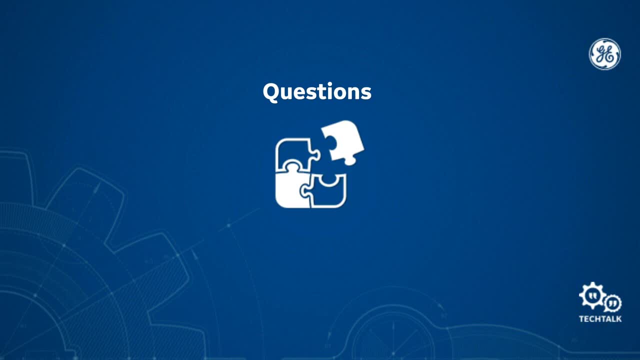 You would do some things with distance elements. You can use also a ground directional overcurrent to help you And, of course, a KV bar to the door. things are going real wrong. high set overcurrent just in case. So, and this is another, 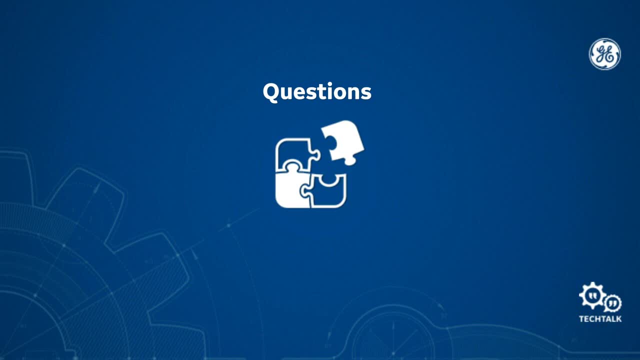 it depends, and really the best way to do series compensated is to look at your line and see where your ETs actually where your VTs are. The VTs are the most important part of this, And so what we're going to do is. examine the fault and where those reactances are. those capacitive reactances are. So if the fault is through some capacitive reactances, we're going to change our reach by subtracting that out of the reach. Yeah, the problem is we don't want to overreach. We need to know where those capacitors are to get our total line impedance to the point where we can deal with it. Another problem with series capacitors in a line- the capacitor bank for series compensation is sub-synchronous oscillations And that can reduce the reach even more.